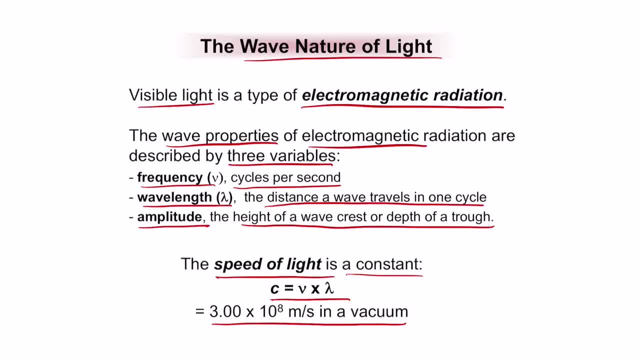 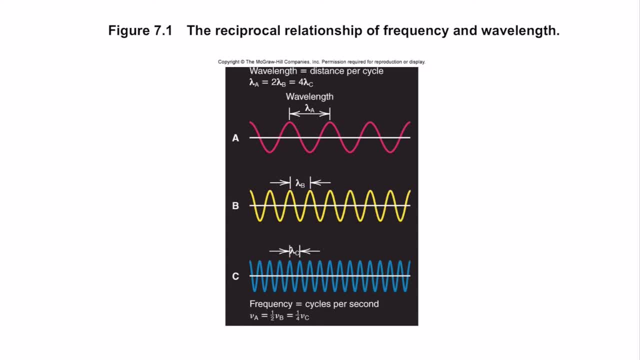 three times ten to the power, eight meter per second. So what is the relationship between frequency and wavelength? So frequency is inversely proportional to wavelength. So when the wavelength is small and the wavelength is large, the frequency is small. When the wavelength is moderate, the frequency is a little higher, And the shorter the wavelength, the higher. 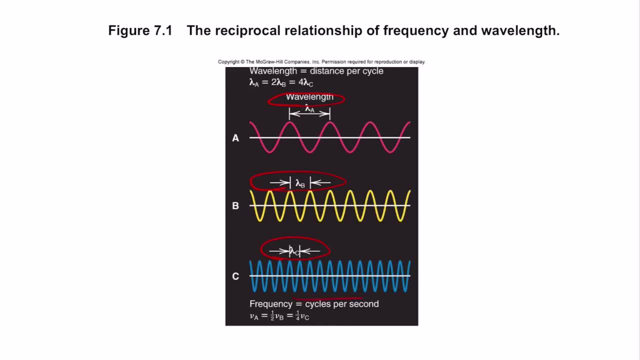 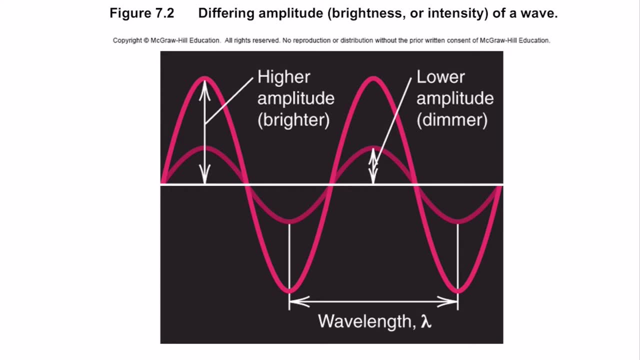 the frequency. So frequency and wavelength have a reciprocal relationship. Now, in terms of the amplitude, what does amplitude generally represent? Amplitude represents the height of the wave. The height of the wave is similar to the brightness: The higher the amplitude, the brighter the light. The lower the amplitude, the dimmer the light. 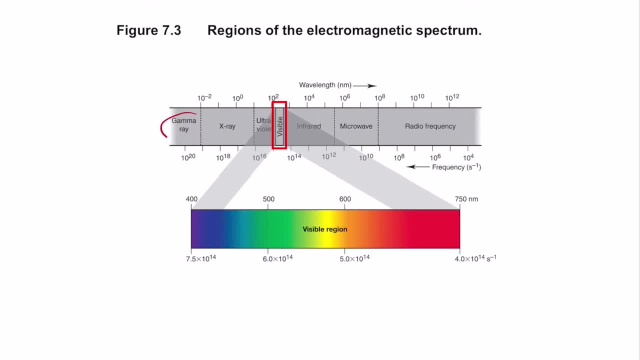 Now. so what is the electromagnetic spectrum? So you start at gamma rays, which have really high frequencies, and you end up with radio waves which have really low frequencies but high wavelength. So visible light can be divided into VGR, So violet, indigo, blue, green, yellow, orange and red. 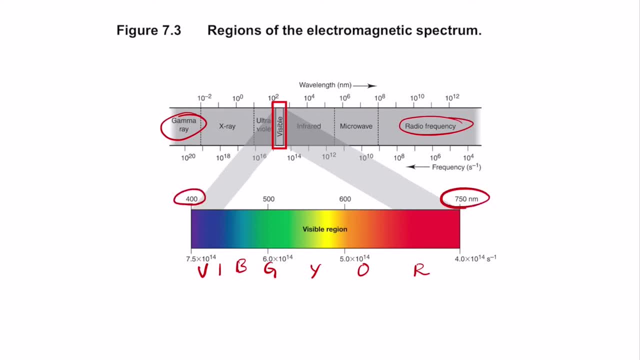 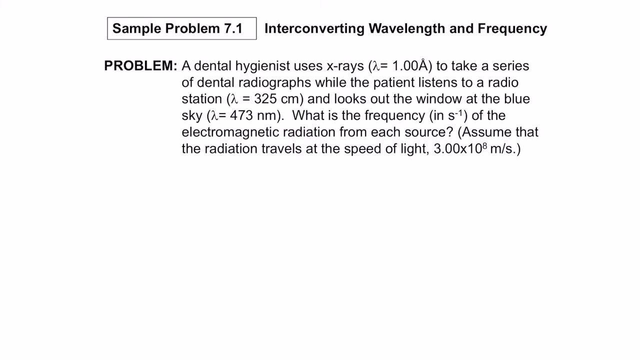 So, and each of them range from around 400 to 750 nanometers. So let's try a problem here where we are interconverting wavelength into frequency. So you have a dental hygienist that uses x-rays with a lambda of 1 Armstrong. 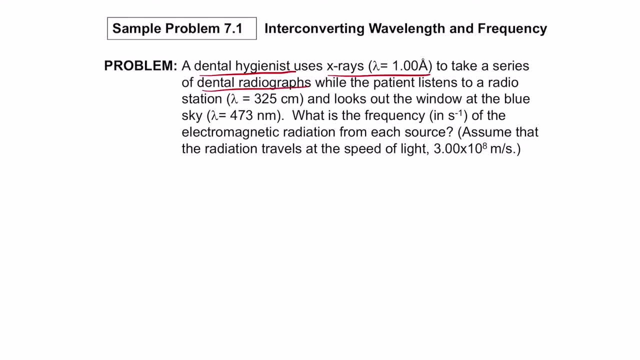 to take series of dental radiographs, while the patient listens to a radio station of lambda 325 centimeters and looks out of the window with a blue sky of 473 nanometers. So what is the frequency of the electromagnetic radiation from each of the sources? 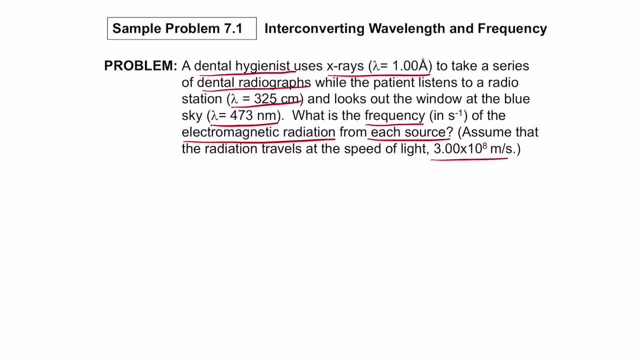 So they have given us the velocity, which is 3 times 10 to the power, 8 meter per second. So we know that C here is the product of lambda times CF. So using this formula we can find every one of these frequencies. So let's start with the first one: x-rays with a lambda of 1 Armstrong. 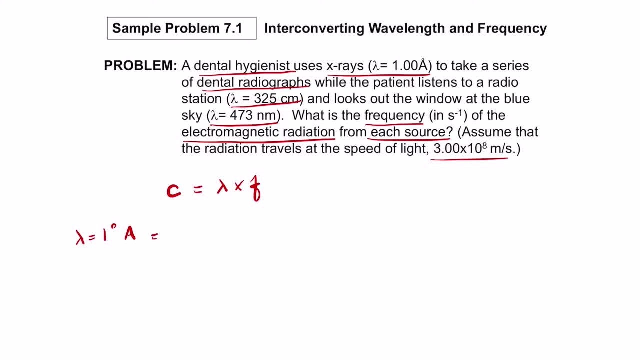 So Armstrong is a unit that represents 10 to the power negative 10 meter Now. so we know that F here becomes C. by lambda C is 3 times 10 to the power 8 by lambda is 1 times 10 to the power negative 10.. 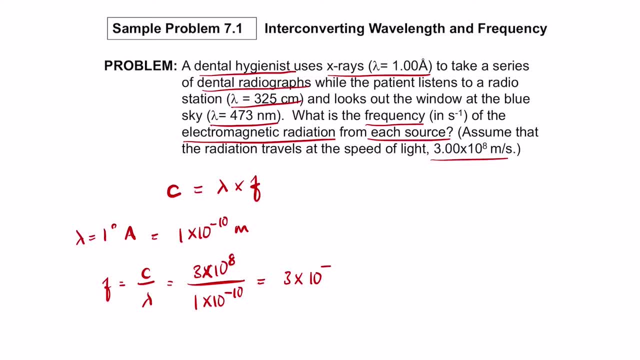 So it becomes 3 times 10 to the power 8 times 10 to the power 10.. So it becomes 3 times 10 to the power 18 hertz. So this is the frequency of the 1 Armstrong, 1 Armstrong. 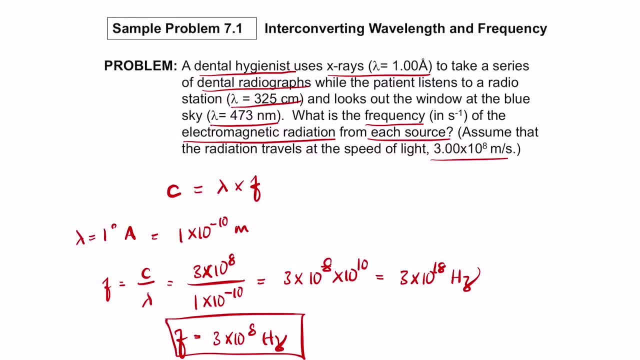 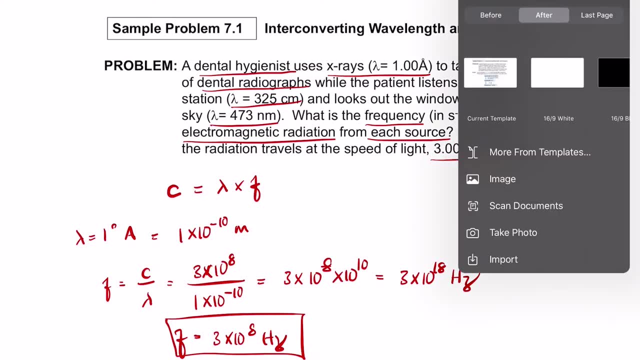 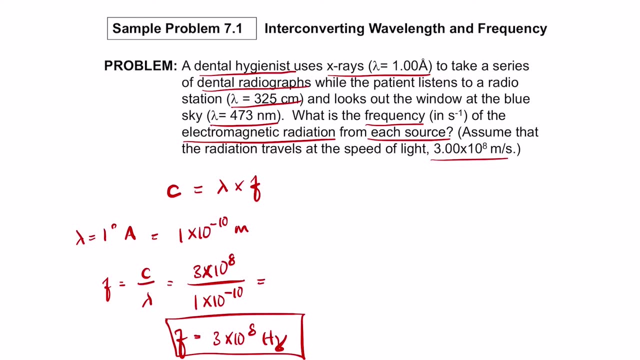 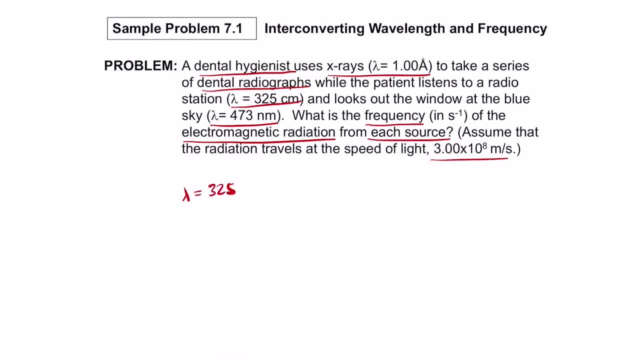 The second one. we have 325 centimeters. Convert it into meters so it becomes 3.25 meters. So we have 3!25 meters, So the F becomes C by lambda. So 3 times 10 to the power, 8 by 3.25.. 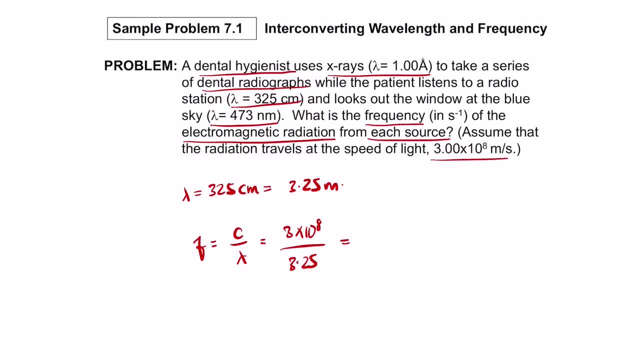 calculate 3 over 3.28. 3 over 3.25, the value is 0.923 times 10 to the power 8. so when you take 110 out you get 9.23 into 10 to the power of 7 Hertz. so this is: 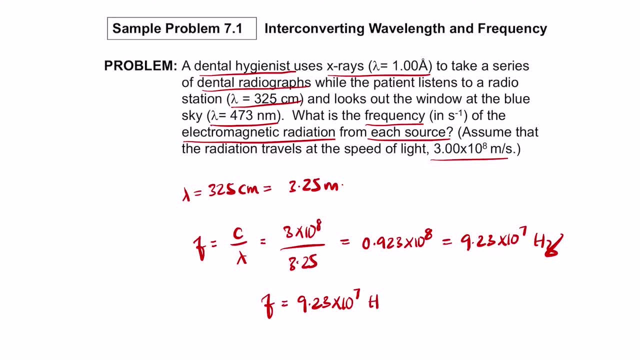 the frequency. this is the frequency of the light that is given here, so this is how you can find the frequency, so using this principle on. next, we have lambda equal to 473 nanometers, so let's try and solve the problem. next one: you have lambda equals 473 nanometers, so 473 nanometers becomes 473 times 10 to the. 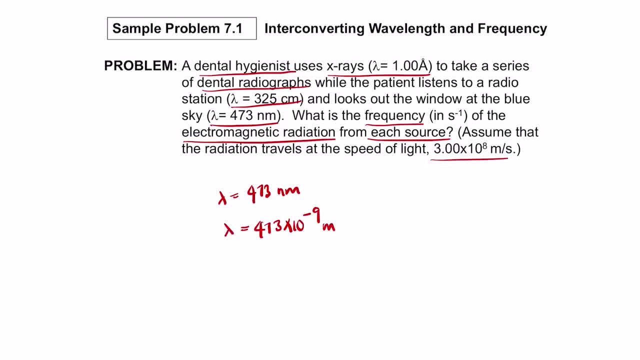 power negative 9 meters, so 1 nanometer is 10 to the power negative 9 meter. so F becomes C over lambda. C again is 3 times 10 to the power 8 by 473 times 10 to the power negative 9, so 3 by 473 times 10 to the power 8. 10 to the power. 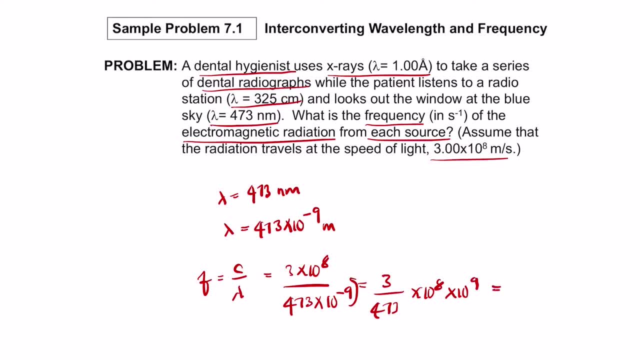 negative 9. when it goes up, it becomes 10 to the power of 9. now let's try and find 3 divided by 473, so the value becomes 0.0063 times 10 to the power 17, so the value becomes 0.0063 times 10 to the power 17. 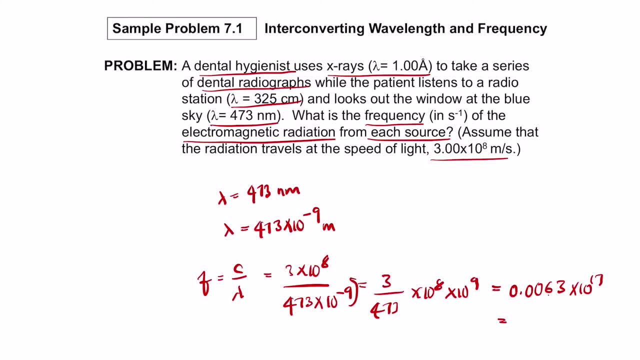 so when you move three zeros here, so this one, here you have to move three places, so 0.0063. so when you move to when you are 10 to the power, 3 here you get 6.3 into 10 to the power. so remove three, three values from the power, so it. 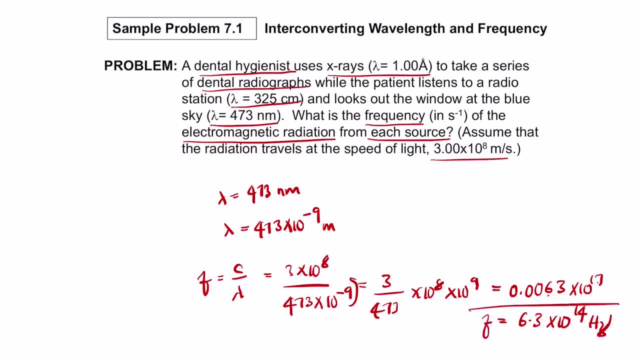 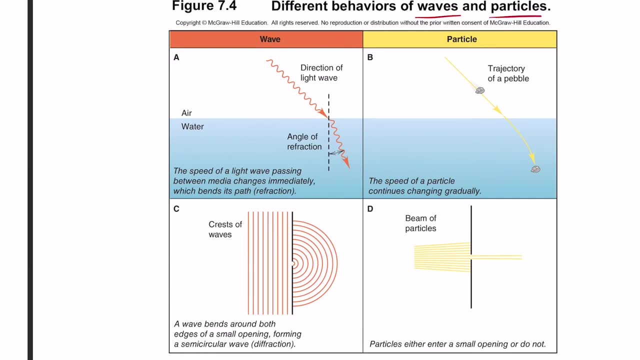 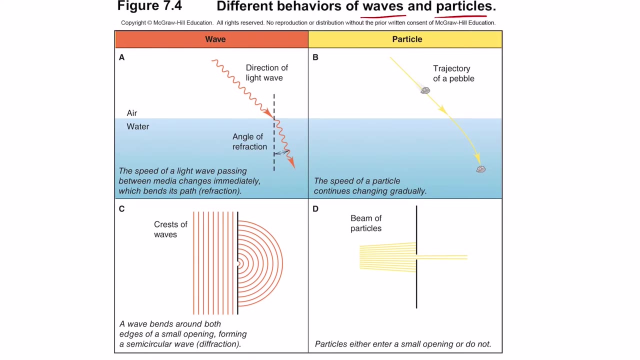 becomes 14 Hertz. so this is the frequency. so this is how you can get all the values using the simple formula F equal to C by lambda. now let's look at different behaviors of waves and particles and how to differentiate the behavior. a wave in general, behaves the same way as a particle. so when you take 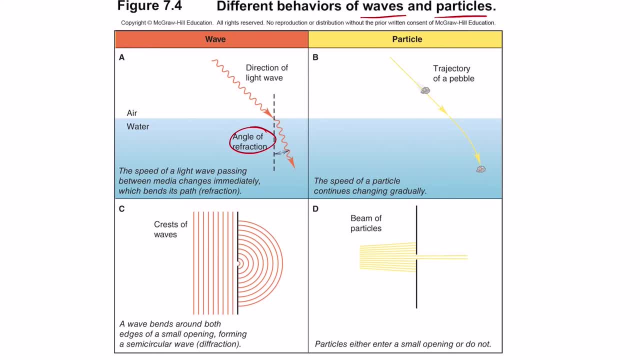 a wave wave generally bends, so creating an angle of refraction, but a particle- particle changes its position gradually rather than changing it suddenly like a wave. a wave would change it suddenly, but a particle changes it slowly. now the same thing when you look at it in terms of waves that are bending around. 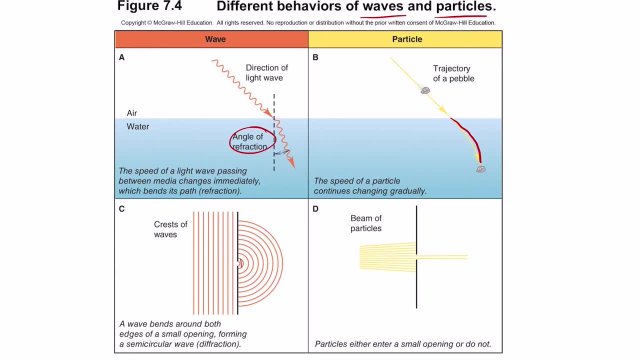 a small opening. when you look at a wave, it creates wave fronts, but when you look at a stream of particles- so think of this- like you know a time-glass- you have a sand glass where sand pours down. when you take sand pouring down, you notice that the particles go in a straight line rather than dispersing throughout the 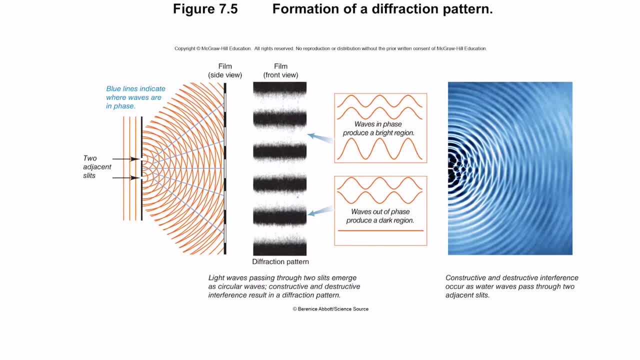 system. so this is the difference in behavior between a wave and a particle. now, the initial idea for light was first conducted by the diffraction pattern that were created by the Young's double slit experiment. when you pass a single source of light, a coherent source of light, through two slits, it creates a 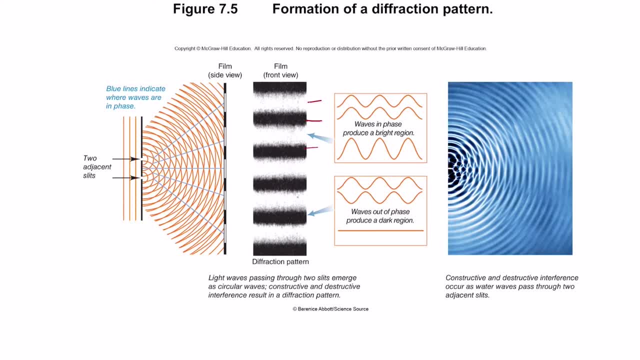 stream of bright and dark fringes. so this bright and dark fringes happen due to constructive and destructive interference. so what happens now? at one point, all the peaks will match. so when the peaks match, it creates a bright fringe. when the peaks collapse, what will happen when they are in the opposite? 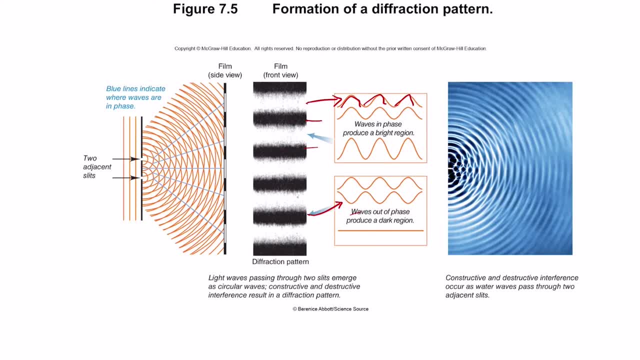 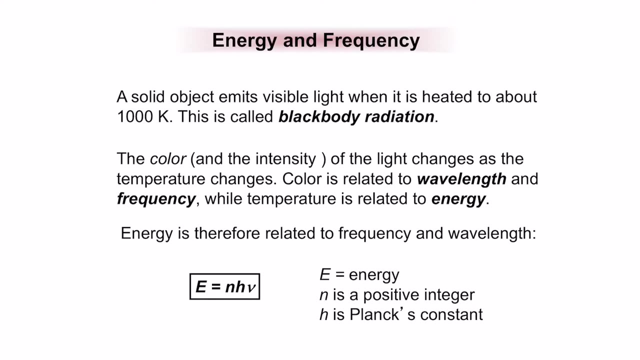 directions, they collapse each other. that creates dark regions. so this series of bright and dark regions, these are called fringes. so this is how the light behaves as a wave. this is what the first discussion of: how light behaves as a wave. now let's discuss energy and 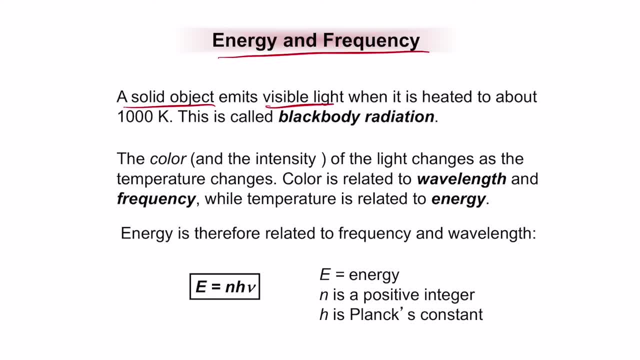 frequency. so a solid object in general emits visible light when you heat it up to a thousand Kelvin. so this here this type of radiation is called as black body radiation. now the color of the light changes as the temperature changes, because color here is related to the wavelength and frequency, while 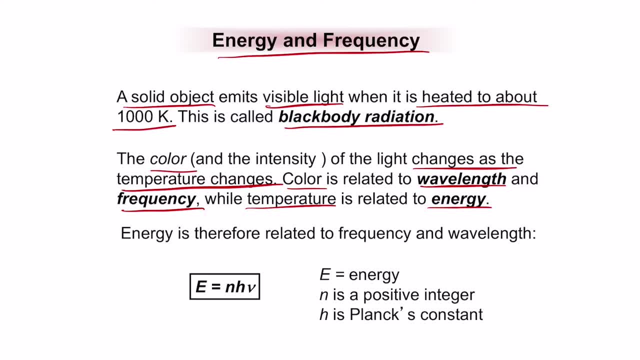 the temperature is related to energy. combining both comes the equation E equal to n, H, nu we also call this the Planck, so we also call this the Planck's law of radiation, or Planck's law of blackbody radiation. where n is a positive integer, H is the Planck's constant. 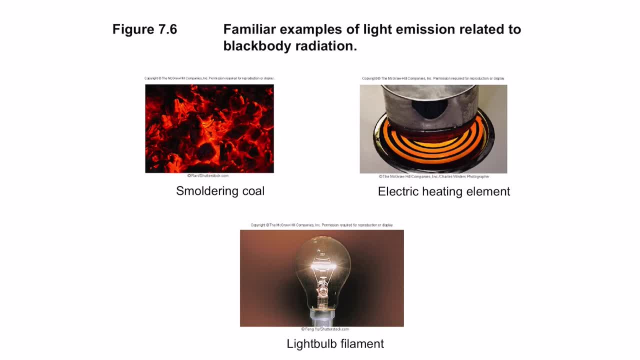 and E is the amount of energy. so this is the experiment that we commonly know: when you heat up something, it produces color: the hotter it is, the more redder it is. so this is a common theme that we can see here. so this brings us to the quantum. 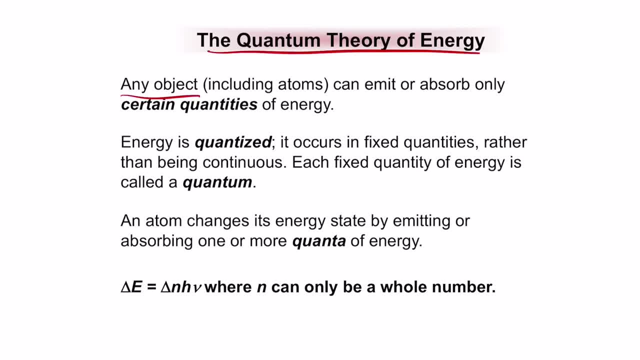 theory of energy. so the quantum theory of energy says that any object can either emit or absorb energy, certain amounts of energy, and this energy comes in terms of packets. we call that quanta, so it undergoes quantization. so quantization occurs in fixed quantities rather than being continuous, and each fixed 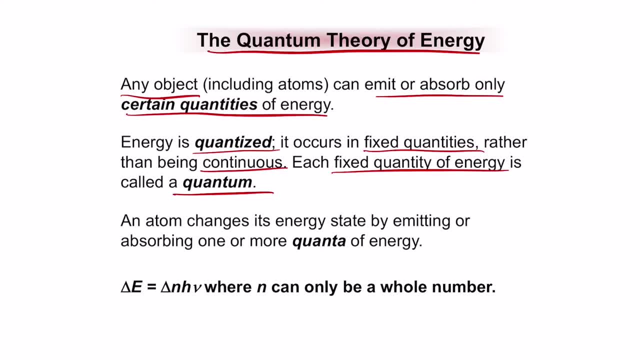 quantity of energy. we call that a quantum. now, an atom changes its energy by emitting or absorbing one or more quanta of energy, so we call this Delta E. Delta E generally is given as the change in energy is even as Delta n times H, nu, where n can be a whole number, only, so n. here is the one that represents the. 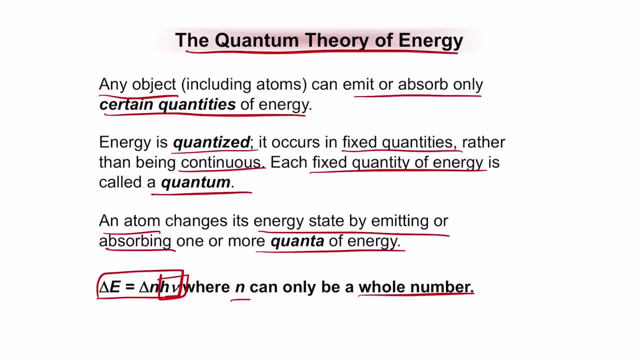 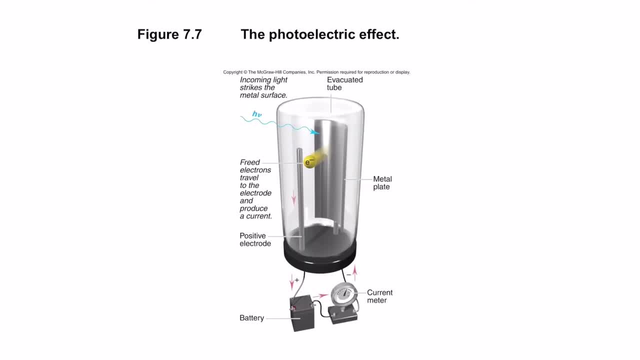 number of particles. H? nu is the energy of each individual particle. so H? nu is the energy of one particle. del nu is the number of particles that change. so this was first shown by the photoelectric effect, so which was first proposed by Einstein. so what did Einstein do? he stroked a metallic screen with 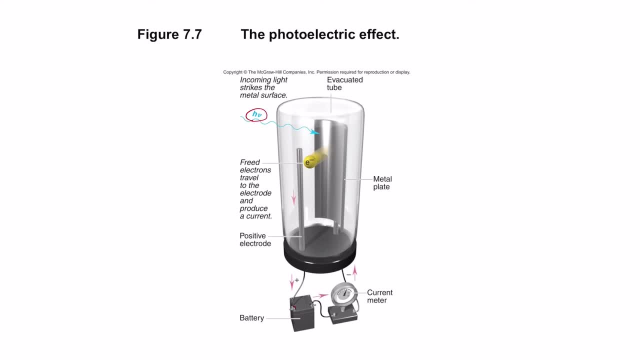 powerful radiation, he noticed that the powerful radiation actually emitted electrons. notice that until then people had the idea that light was a wave and Newton, using his photoelectric experiment, he proved that even as a wave it can have energy and that individual energy particles are called photons. so this is 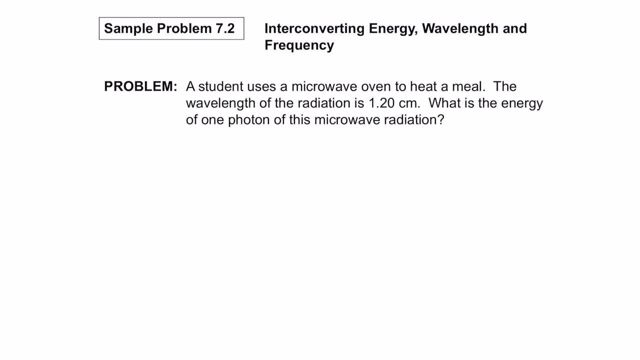 the first term the name comes through. so let's take an example. you have: a student uses a microwave oven to heat a meal. the wavelength of the radiation is 1.20 centimeters. what is the energy of one photon of this microwave radiation? so the formula is E equal to n, H, nu, so the value for H is 6.63 into 10 to the. 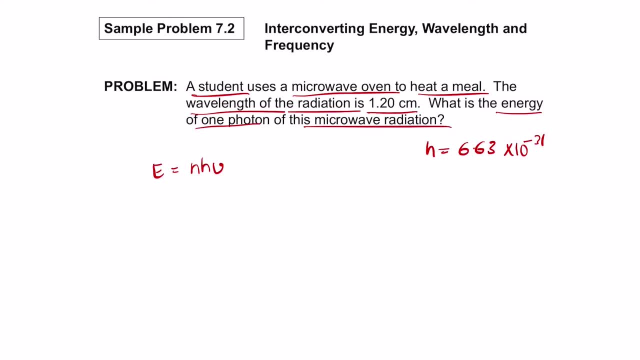 power negative 31- sorry, 6.626 into 10- to the power negative 31 joule second. so this is the value of Planck's constant. remember the value for Planck's constant now? so, with this into consideration, now we have one proton, one photon, so which? 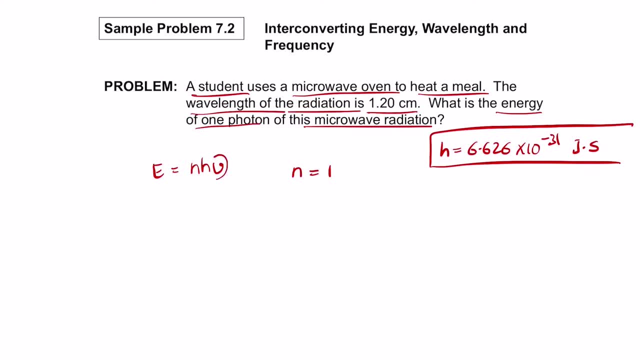 is n equal to 1, and we'd know, we have to know the velocity. so how do you find the velocity? so they have given that this is a microwave oven, so which means that it is still microwave radiation. microwave radiation also travels at the speed of light, so nu, here is not velocity, but nu here is actually the frequency. 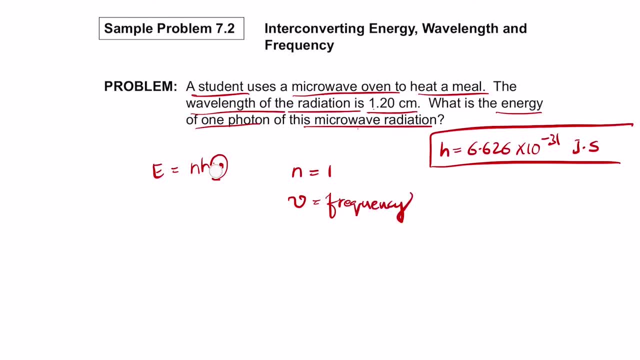 so remember that nu here represents the frequency. it's not v actually, it's a curved v, v. so v here represents the frequency. but they have given us the wavelength. wavelength is given as 1.20 centimeters. convert it into meters, you get 0.012 meters. 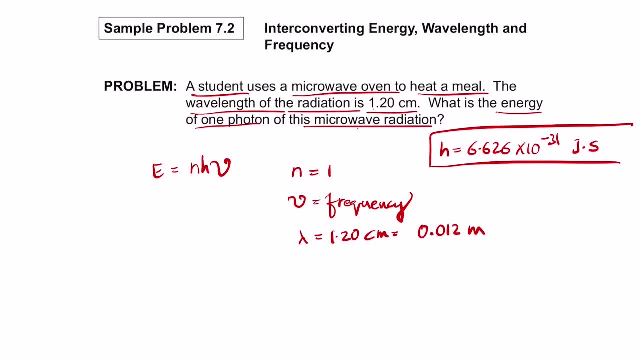 now, with this into consideration, what can we write here? we know that nu here is c by lambda, c here is 3 times 10 to the power 8 by 0.012. so 3 divided by 0.012 becomes 250 times 10 to the power 8, so we can write it as 2.50. 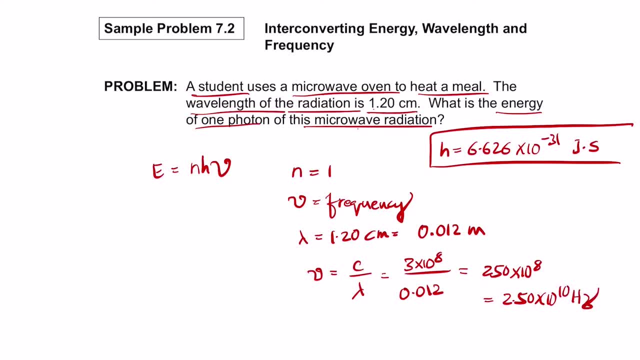 into 10 to the power of 10 hertz. so substitute the values into the formula. so e is 1 times h is 6.626 into 10 power negative 34. sorry, this is 34 times 2.50 into 10 to the power of 10. 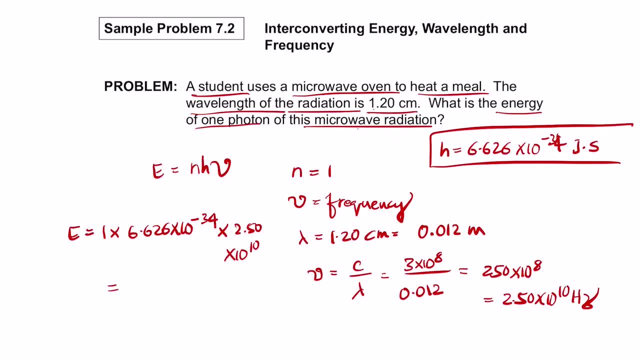 so, using the values now, you have 6.626 into 2.50, so it becomes 16.565 times 10 to the power negative 34 times 10 to the power negative 10 gives you 10 to the power negative 24.. so when you can write this, if you can write it like this: 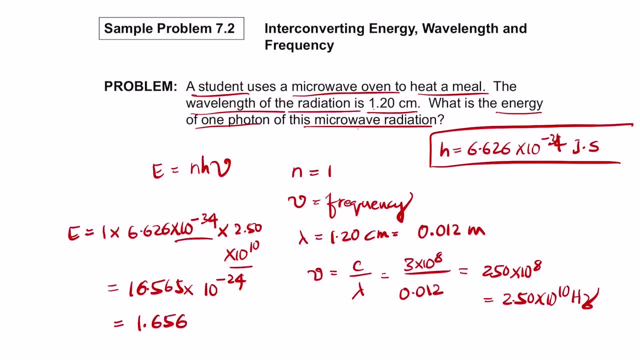 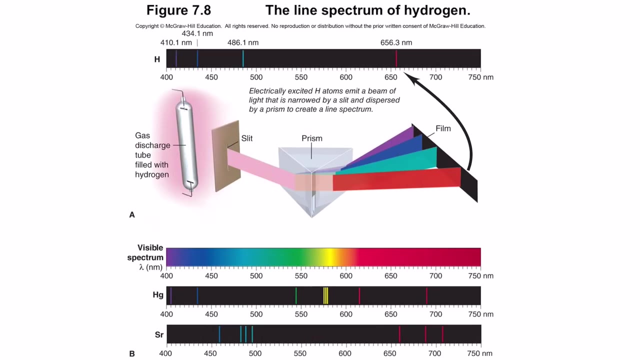 we can write 1.656 times 10 to the power of negative 23 joule. so this is the value of energy of that particular particle, one photon of the microwave radiation. this is the amount of energy that each photon carries. now, next let's talk about atomic spectrum. so when you pass 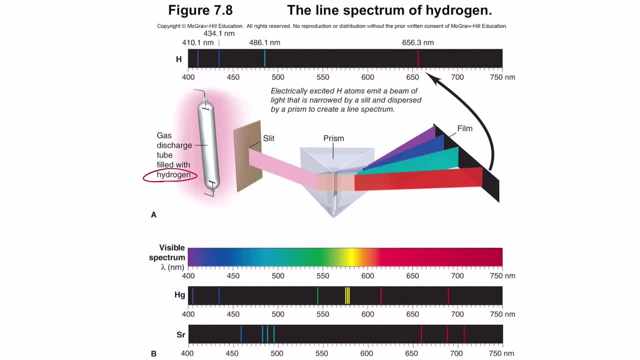 a laser beam on hydrogen and heat it up to a certain temperature. we know that every body, when you heat it up, it releases radiation, so the radiation that is emitted by hydrogen is generally classified under the spectra, under the visible spectrum. you can see that you have four different wavelengths that are generated: 4, 10 nanometers, 434, 486 and 656. so why does this happen? 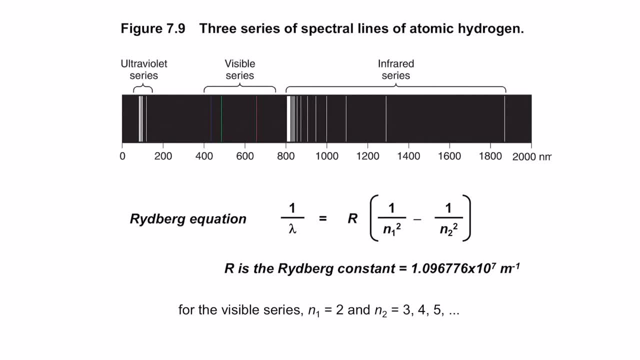 and how can you explain this? radiation and the wavelength can be explained by the Rydberg equation, which can be written as: 1 by lambda equals r times 1 by n1 square minus 1 by n2 square, where n1 is the first energy. 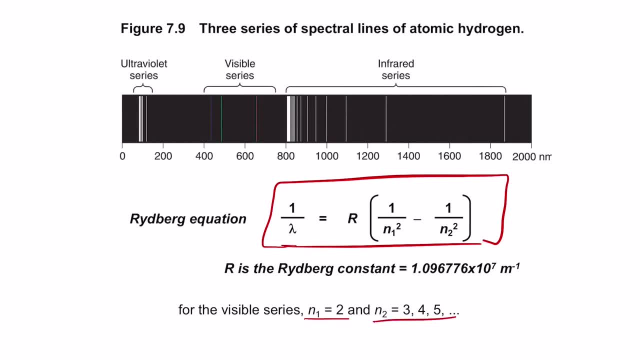 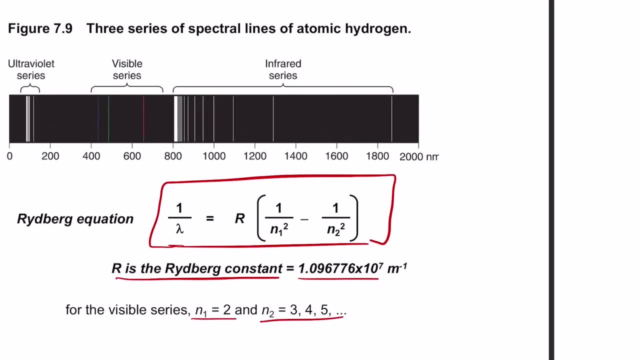 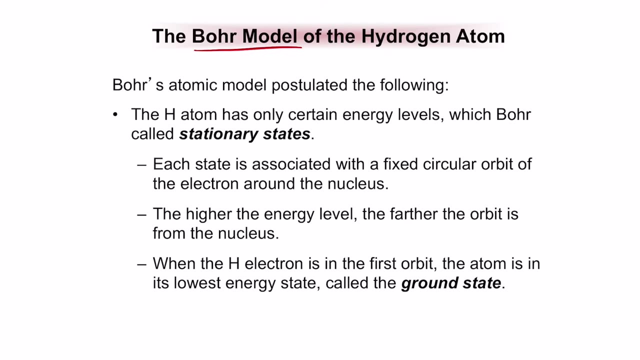 level ground state, and n2 is the higher energy levels. r here is as the Rydberg constant, which is 1.096776 into 10 to the power of 7 per meter. so this was first explained by the Bohr's model, so Bohr's atomic model. so Niels Bohr first postulated the idea behind why the atomic 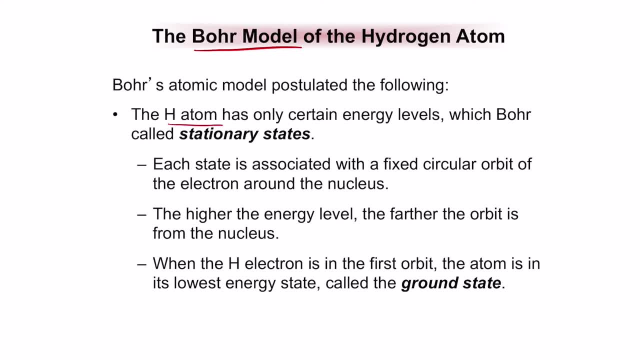 spectra exists. so he postulated that the hydrogen atom has only certain energy levels and he called it the stationary states, and each state is associated with a fixed circular orbit and the electron around the nucleus, and the higher the energy level, the farther the orbit is from the nucleus. now, when the hydrogen electron is in the first orbit, the atom is in its lowest. 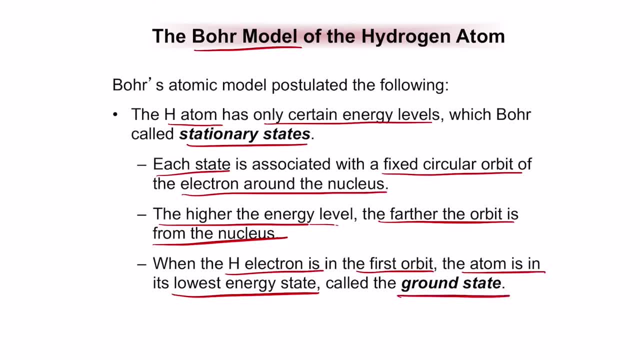 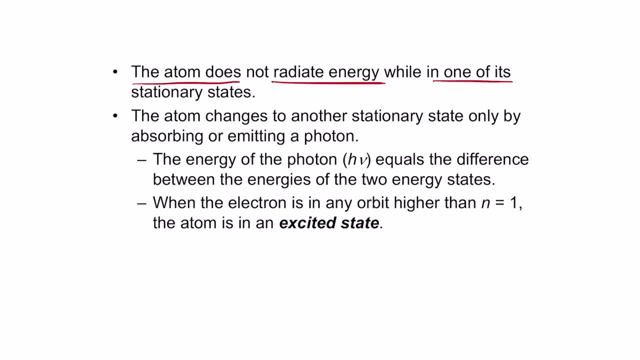 energy level, and the electron is in its lowest energy level. and the electron is in its lowest energy state. the atom that is in the lowest energy state is called as the ground state. now, the atom will not stay the same way, so does not radiate energy, while one of its stationary states. what? 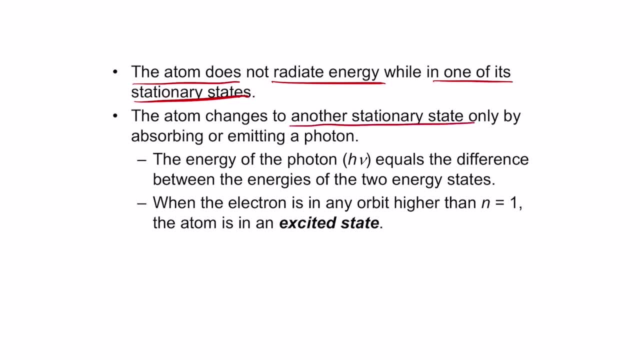 will happen is that when it changes one state to the other state, it either does it by absorbing or emitting a photon. now, the energy of the photon equals the difference between the energies of the two electric energy states, so the when it jumps, when it goes from a lower energy to a higher, 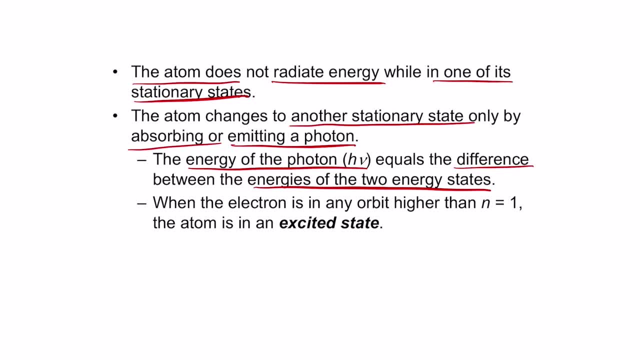 energy. it absorbs energy when it comes back from a lower energy state. it does not radiate energy. when it comes back from a higher energy to a lower energy, it releases energy. now, when the electron is in any orbit higher than and equal to one, we call that an. 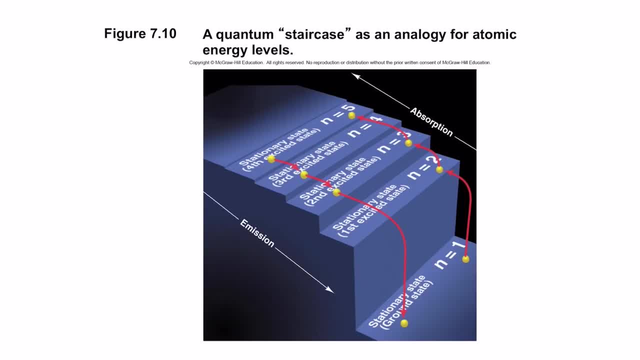 excited state, so remember this term: excited and ground states. so what happens here in terms of the absorption spectrum and emission spectrum, when the electron jumps from the first orbit to the second orbit, and it really it absorbs some energy from the second orbit to the third orbit. it also 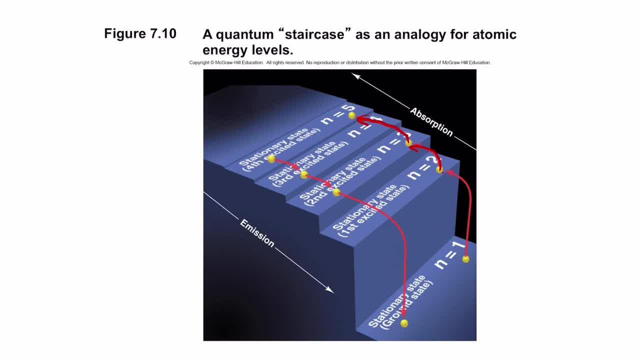 absorbs some energy. from third orbit to the fifth orbit, it also absorbs some energy. the same thing thing happens in reverse as well. in reverse it undergoes emission where from fifth state to fourth it can release energy. fourth through third, releases energy. third to ground state also releases. 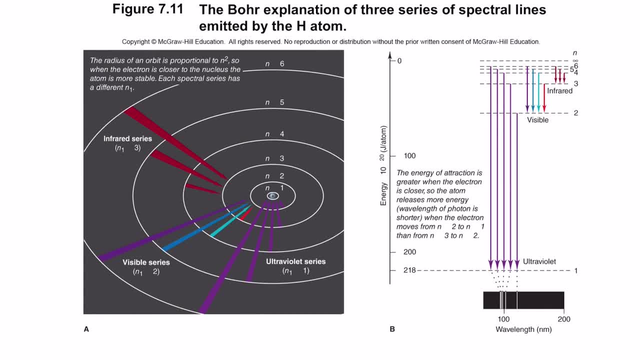 energy. so this energy release is what we consider as the atomic spectrum. so remember that we are initially heating up the hydrogen gas. when you heat up hydrogen gas, what you are doing is basically giving it energy. now, once you remove that heating up, it starts losing energy. that losing is converted. 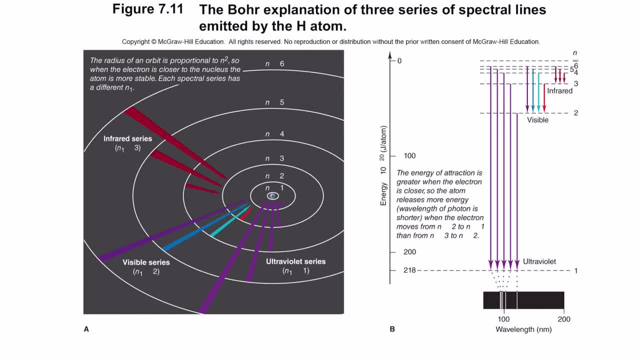 into emission spectrum. now, if the energy level directly falls from the highest energy state to the ground state, the radiation that is really emitted is ultraviolet radiation. so when you go directly into the ground state, you release ultraviolet radiation. when directly you go into the second energy state, that releases visible radiation. when you directly come to the third, 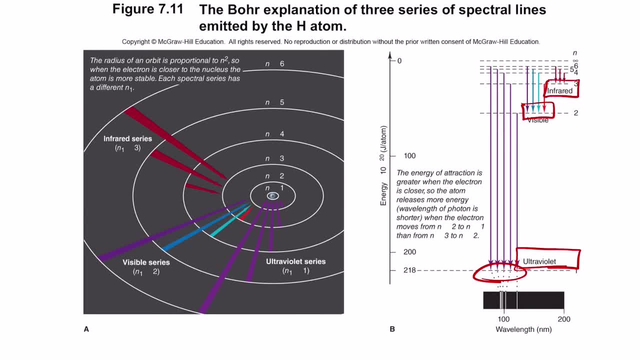 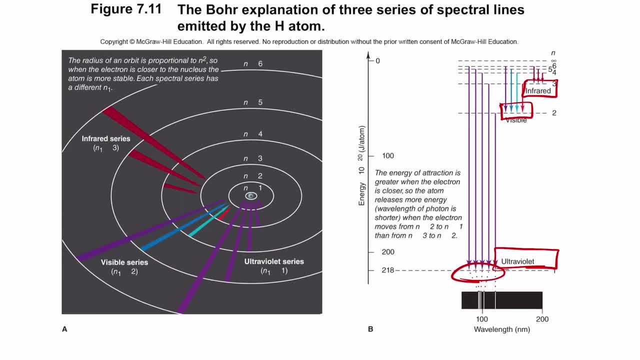 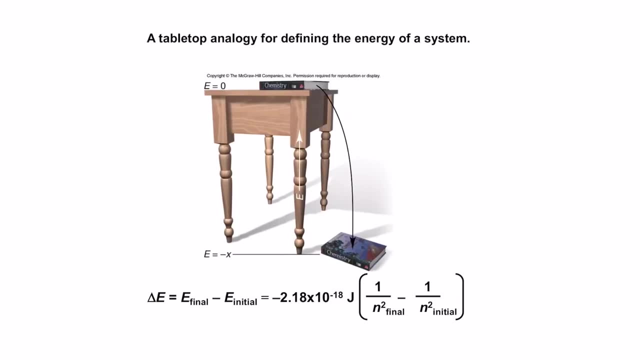 energy state you release, it releases infrared radiation. so this here was given what we call series of names. so these series as Palmer series, a Leiber series, so Lyman series, these are part. you know these are some of the common names given. now, the idea was that when 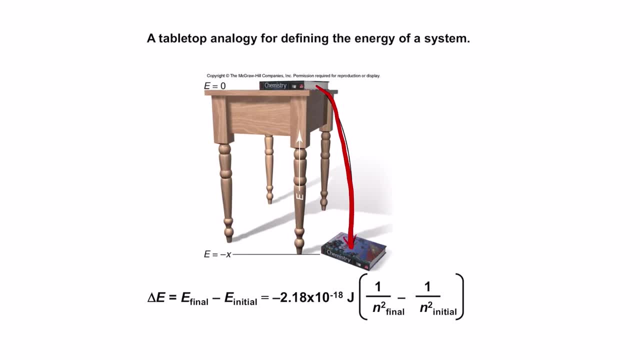 the textbook here. think of textbook falling from a higher state to a ground state, which means that there is an energy difference. that energy difference can be calculated as Delta E equals E final minus E initial, which is given by the formula negative 2.18 times 10 to the power. 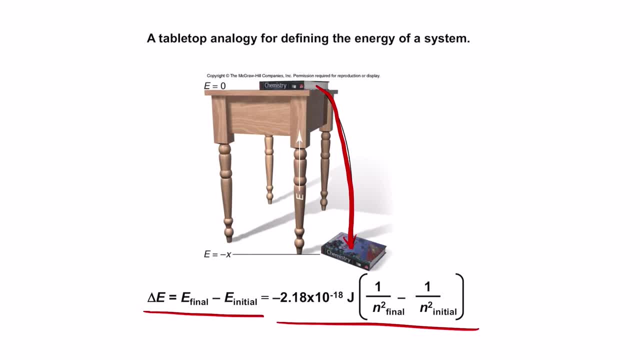 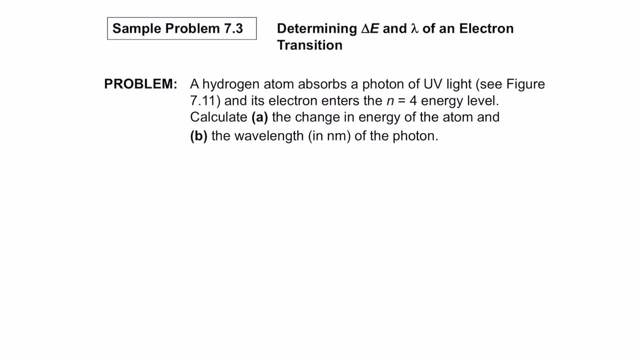 negative 18 joule times 1 by n final square minus 1 by n initial square. so let's try this problem and see if we can use those formulas and write down the problem here. so hydrogen atom absorbs a photon of UV light and its electron enters the 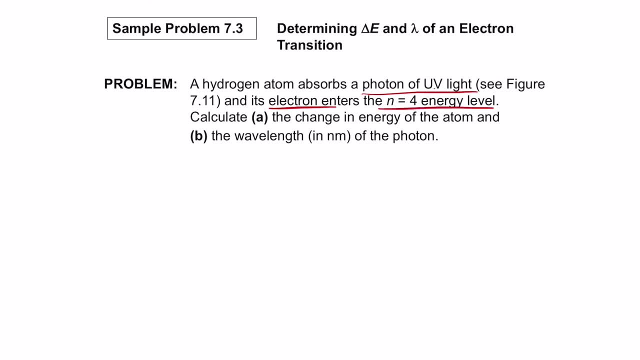 n equal to 4 energy level. now remember that when it absorbs UV light, you are starting from the ground state. so remember that, depending on the type of radiation, you will know where you are starting. so here you are going, from n equal to 1 to n equal to 4. now, first thing they're asking: 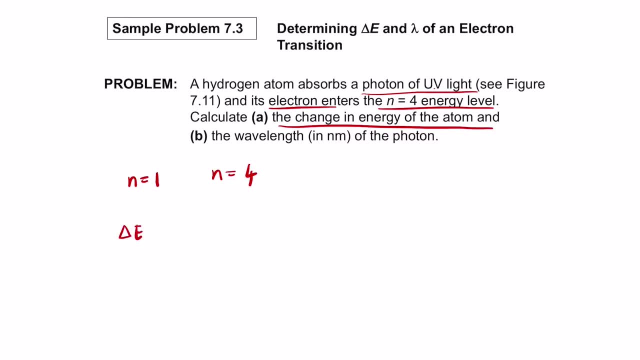 another thing about 18 Joules. that includes W and there's가는. this caught us is that you will have 50, so gets 4 E and, as I said, we can get 8 KM, which is the total energy of the electron, and, as you can see in this picture, we have again about 100 M squared over 20 KM. 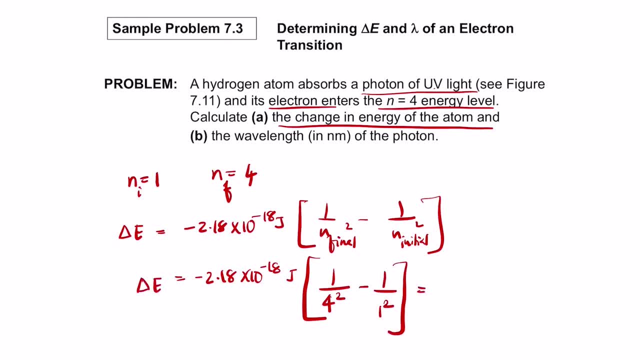 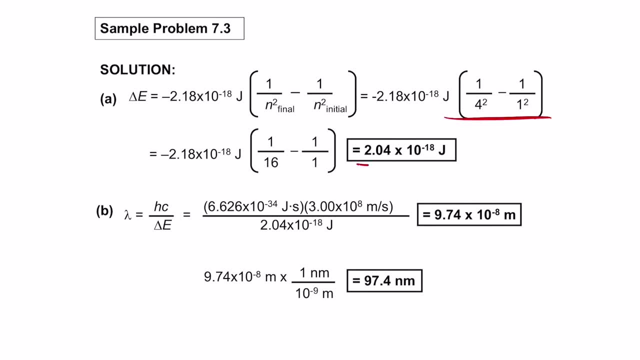 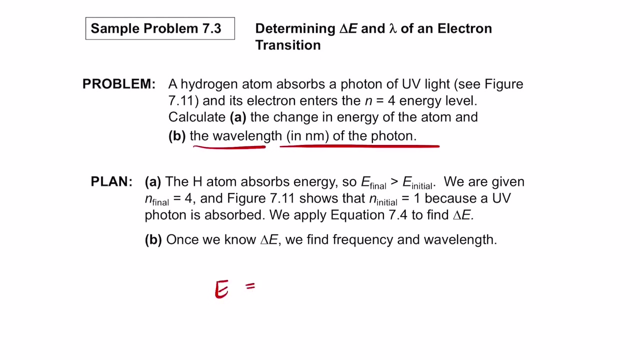 1 square. so when you calculate the value so you should get a value of 2.04 times 10 to the power negative 18 joule. so this is the amount of energy. now how do you find the wavelength here? so we know that the formula for e is so delta. e is delta n times h nu. 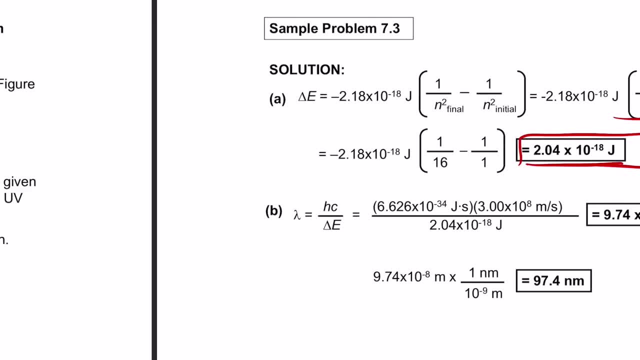 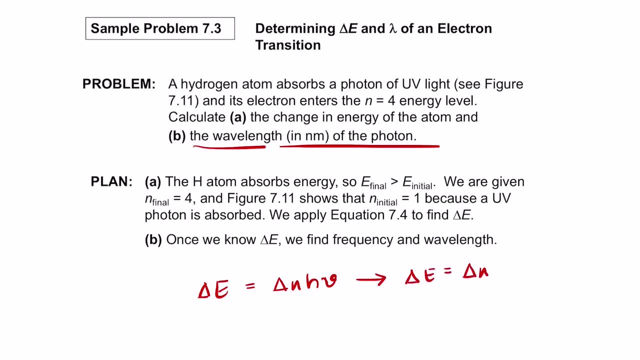 so we are finding the lambda value, so we can replace nu with c by lambda. so delta e becomes delta n times h into c by lambda. so lambda becomes so delta n times hc by delta e. now here we are talking about one single photon, so delta n becomes negligible. so we can simply: 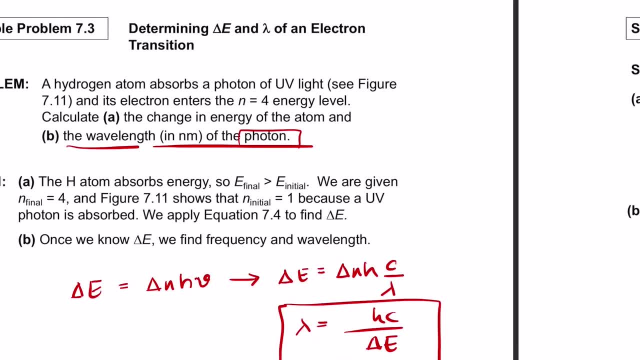 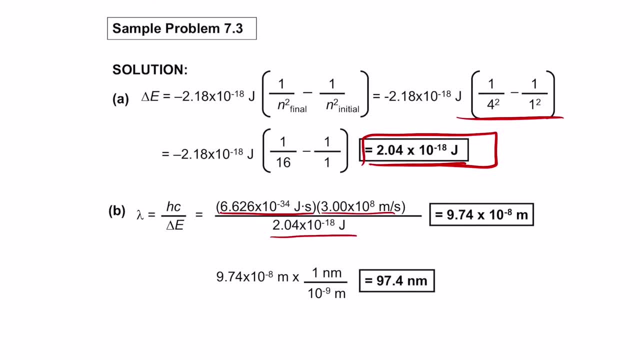 write the formula as: delta lambda equals hc by delta e, so hc by delta e is equal to delta e. h is 6.626 into 10 to the power negative 34. c is 3 times 10 to the power 8 divided by delta e is. 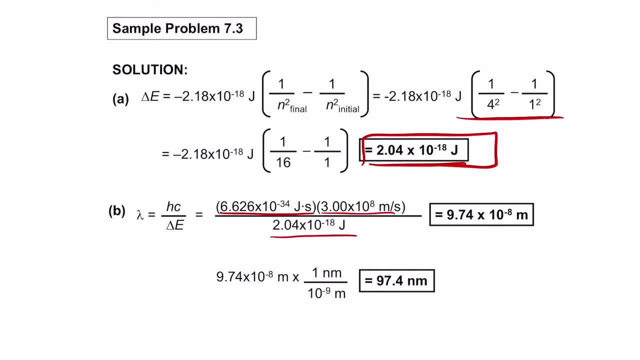 2.04 into 10 to the power negative 18, so which, when you calculate, you end up with the final answer: 9.74 into 10 to the power negative 8 meters. when you convert it into nanometers, it becomes 97.4. 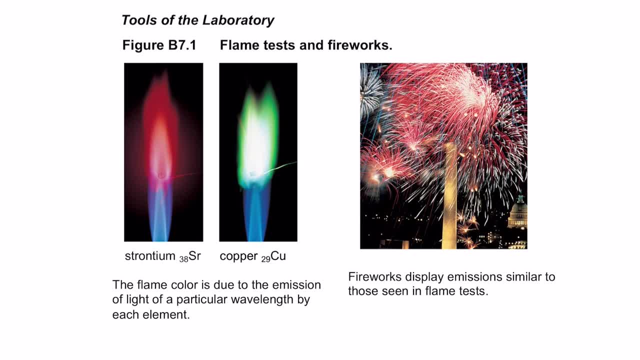 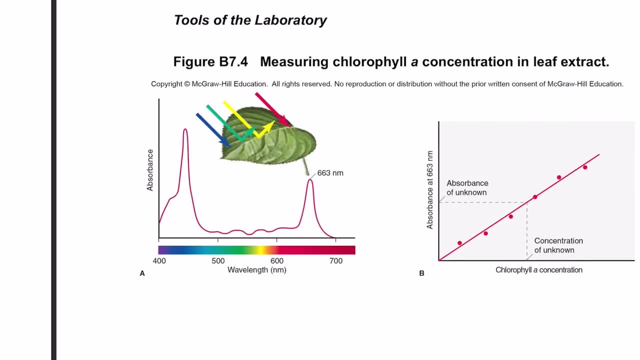 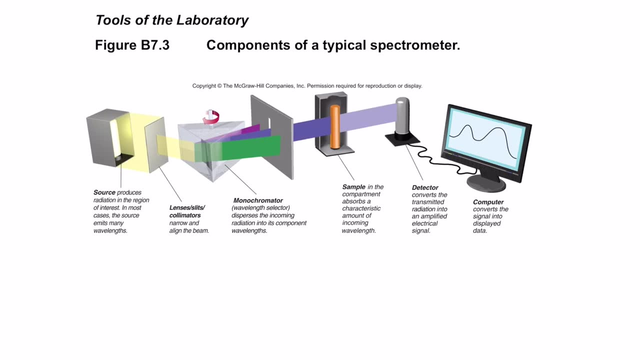 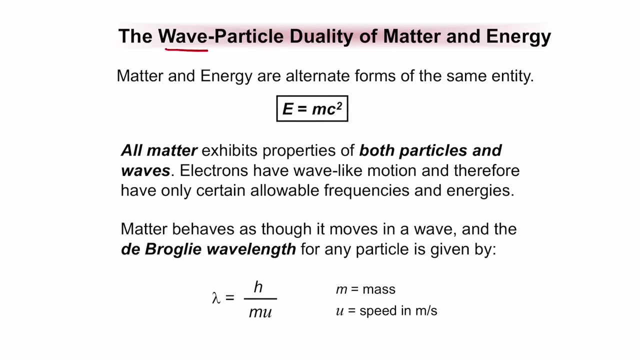 nanometers. so that is how you know that the emission is a uv radiation. so the most common way to measure an object by using its spectrometry, by using a spectrometer. so a spectrometer is the way by which we determine different objects: atomic spectrum. now let's talk about the next topic, the wave. 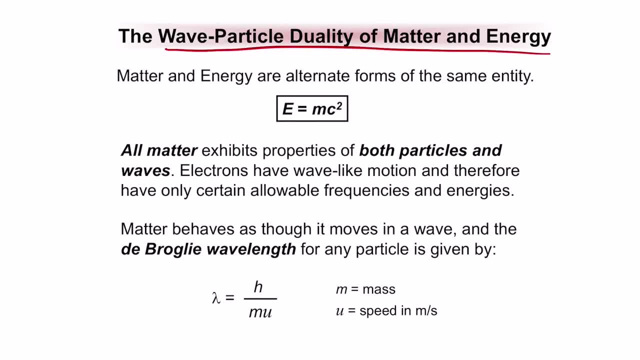 particle duality of matter. so matter in its original state has two different existence, two alternate forms. so matter and energy are alternate forms of the same entity. so they are the same entity but they have different forms. the forms here refer to the wave particle duality, the first equation that was given here. 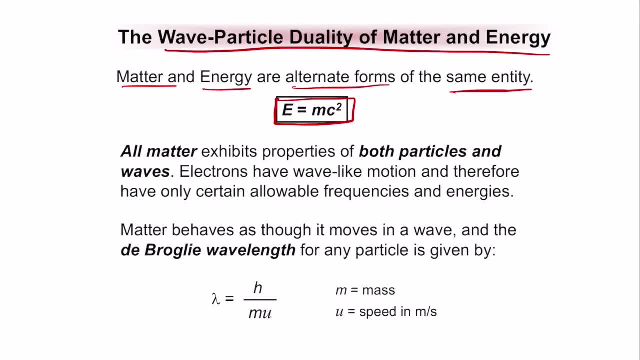 so all matter exhibits properties of both particle and waves. so the first experiment that proved this was electron diffraction experiment. even electrons have wave-like motion and therefore they have only certain allowable frequencies and energies. that was first given by the de broglie hypothesis, which basically stated that every particle has 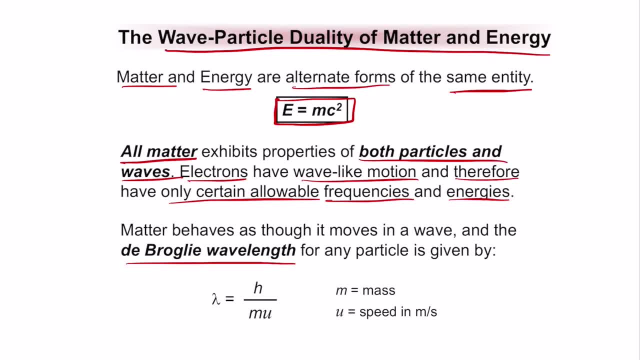 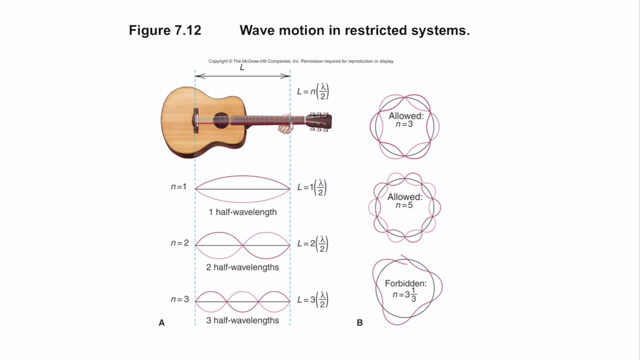 both a mass, and so it behaves as a, both as a particle and a wave. so that he mentioned that the wavelength of that particular particle can be written as lambda equals to h by mu, where m is the mass and u is the speed of the particle. so what are the wave restrictions that it can have? for example, it's allowed to: 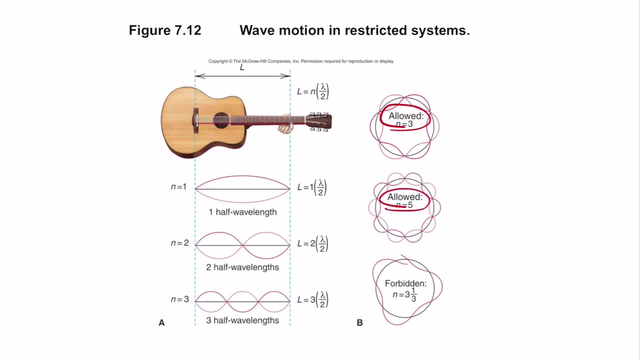 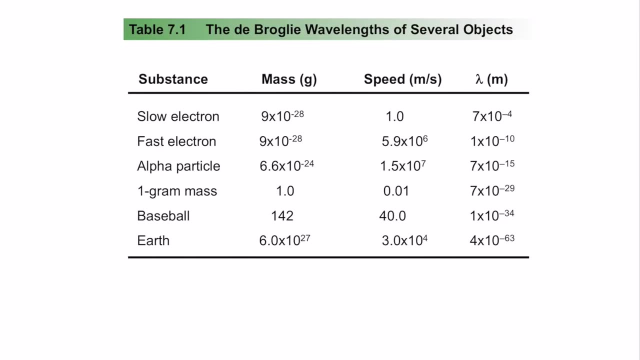 have a n equal to 3, it's allowed to have a n equal to 5, but it is not allowed to have a n equal to 3, 3, 1 by 3. so waves here, wave motion here, is in restricted systems. so a slow electron would have a lambda value of 7 times 10 to the power negative. 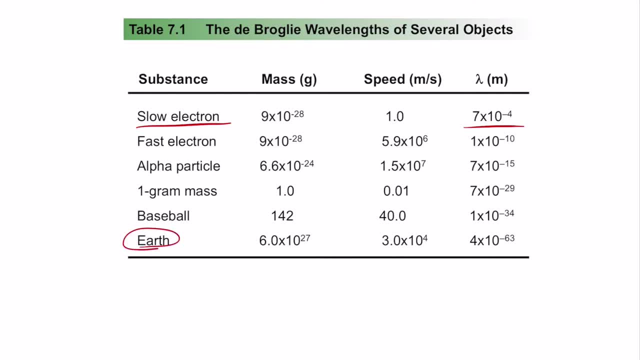 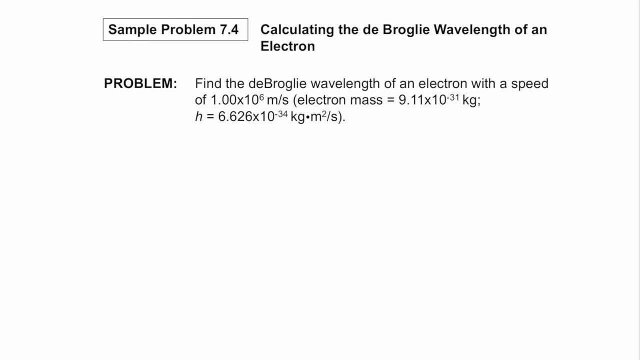 4, but earth because of its big mass and less velocity and high mass results in a lambda value of 10 power negative 63 meters, which is very, very, very low. so this is the idea behind de broglie wave. so use the principle here, so you have everything given. 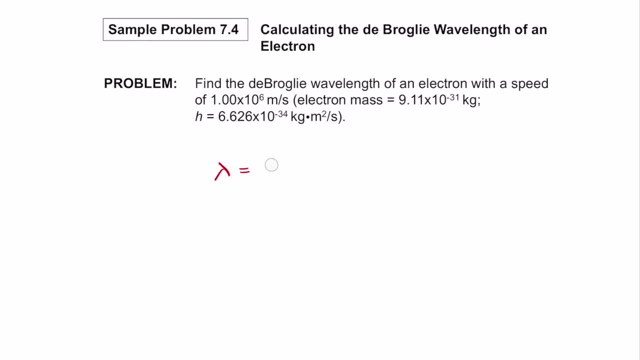 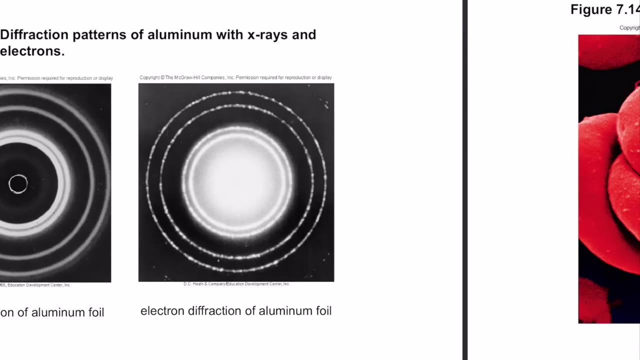 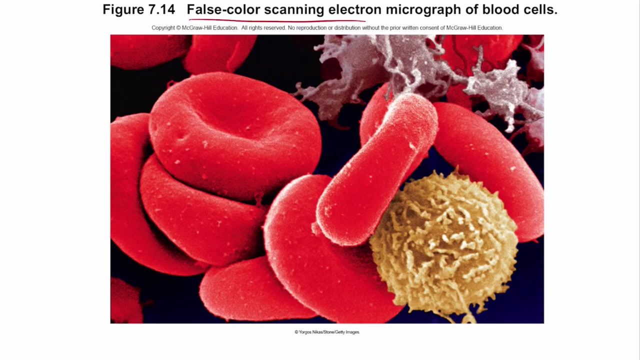 to. so one of the primary uses of using this was the first time- is to use false color electron microscope, micrograph of blood cells. so electron microscopy was first discovered by using this principle of the idea that you can reflect electrons as waves. you can use electrons as waves because they behave as waves. they can also, you know. 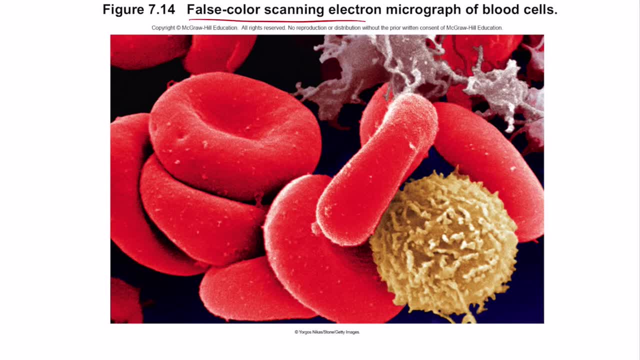 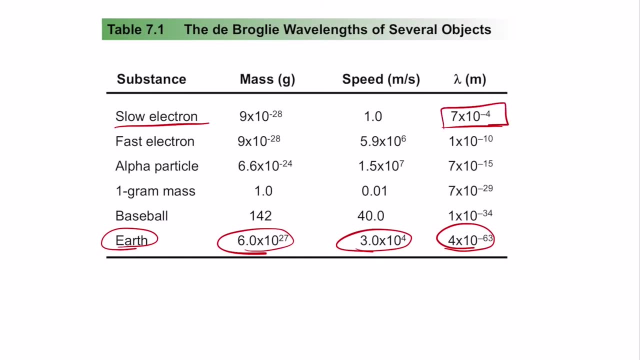 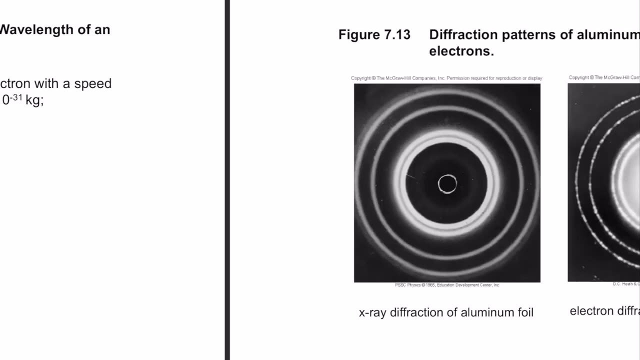 end up becoming a good substitute for light rays and because of the wavelength that that electrons have, because of the wavelength range that the electrons can operate, until fast electrons can operate, until we can use these to look at really, really, really detailed images of objects. so this is an example of 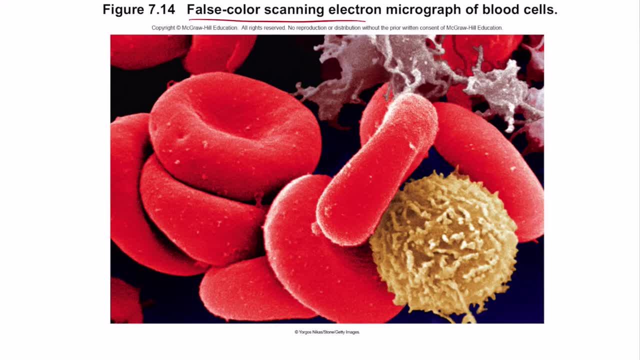 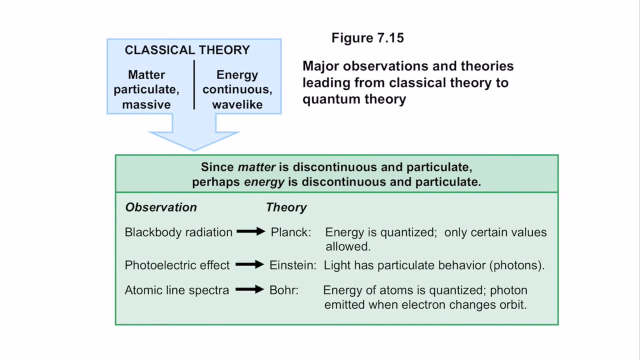 electron microscope, microscopy used to create this kind of ideas. now, what are the major observations and theories leading from classical theory of light to the quantum theory was? the first observation was blackbody radiation by Max Planck, where he said that the energy is quantized and only a 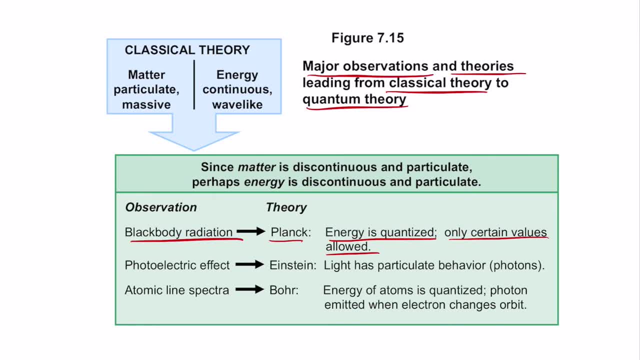 certain values are allowed and you should only get it in multiples. the second was the photoelectric effect observed by Albert Einstein, where he said that light has also particulate behavior and behaves as photons, and you have atomic line spectra, proposed by Niels Bohr, and where he said that the 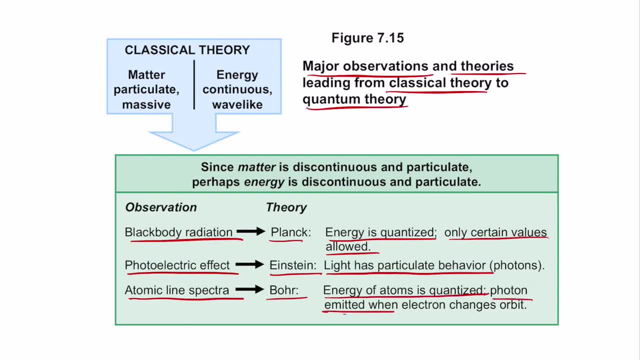 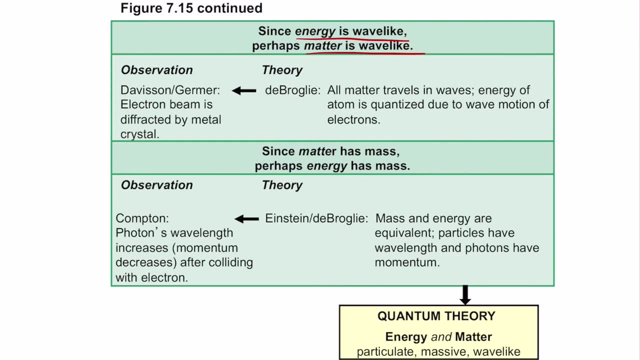 energy of the atoms is quantized and the photon emits when electron changes objects. now, since energy is wave-like, perhaps matter is also wave-like. so the observation was that the electron beam is defected by a metal crystal proposed by the Broglie. so de Broglie basically stated that all. 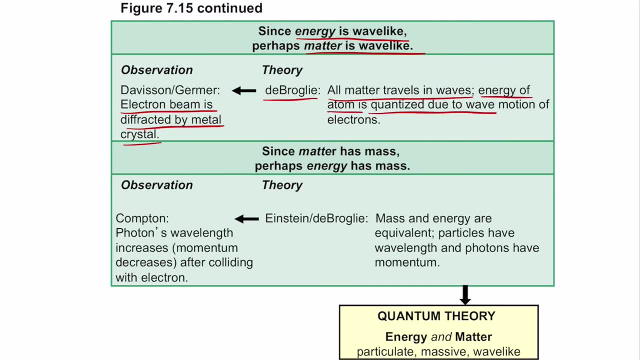 matter travels in waves and energy of the atom is quantized due to the move motion of electrons. now, since matter has mass, perhaps energy also has mass, which was proposed by Einstein and de Broglie, where he used the famous Einstein distractions as equal to MC squared, so where he said that up already a body of a certain mass. 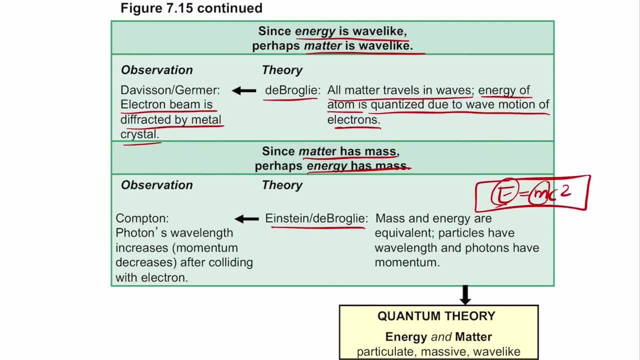 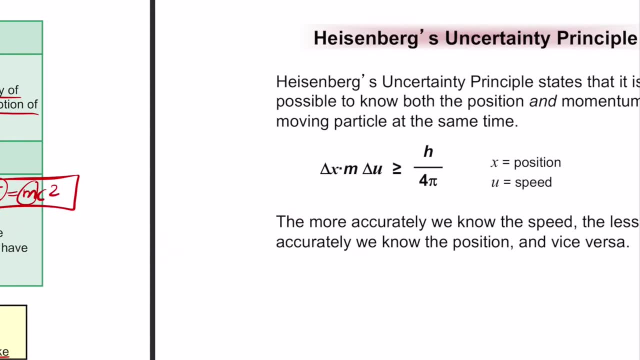 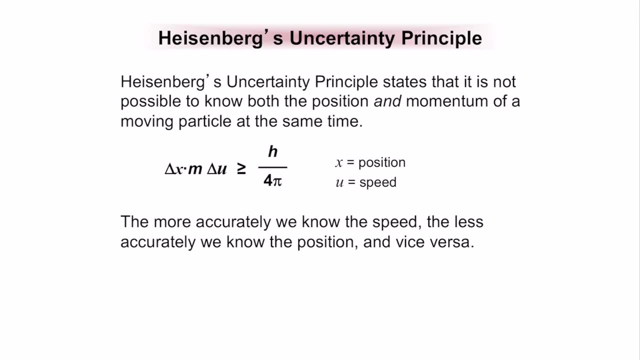 will also have a certain amount of energy. So this gave rise to the quantum theory and where energy and matter are particulate, massive and also wave-like. So because of this problem here this brings up a big problem of uncertainty is that when you are able to follow through and understand the uncertainty, 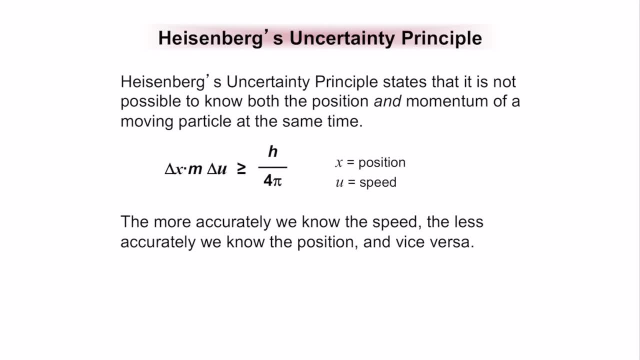 here. what is the uncertainty? here is uncertainty is the amount of error that you get when you are trying to calculate one value and the other value cannot be calculated easily- Now a body traveling. so Heisenberg's uncertainty principle was the solution to explain this uncertainty. It states that it is not. 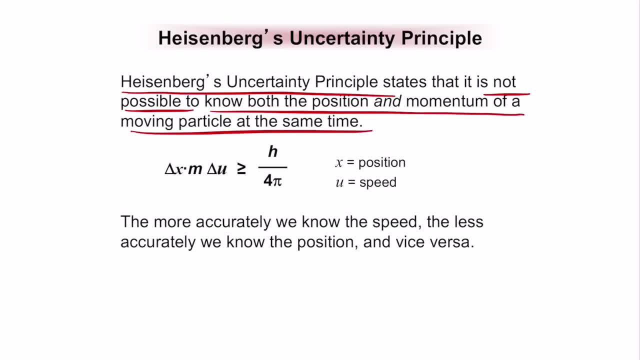 possible to know both the position and momentum of a particle moving at the same time, moving particle at the same time. So there is only one chance: either you can calculate the position or you can calculate the velocity, but you cannot calculate both of them at the same time with high accuracy. So what is? 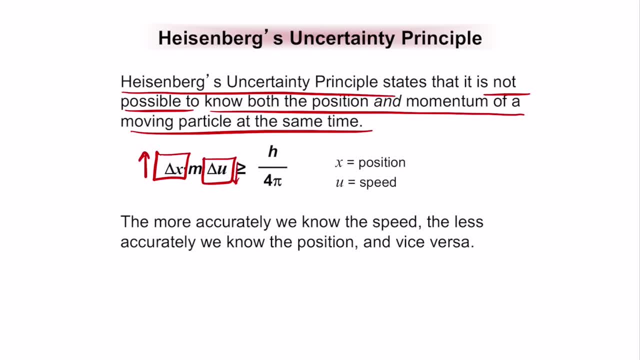 basically saying is that if you want to increase the accuracy of position, then you can decrease the velocity of the particle and you can decrease the accuracy of the velocity. If you increase the accuracy of the velocity, it decreases the accuracy of position. So this was perfectly stated with the 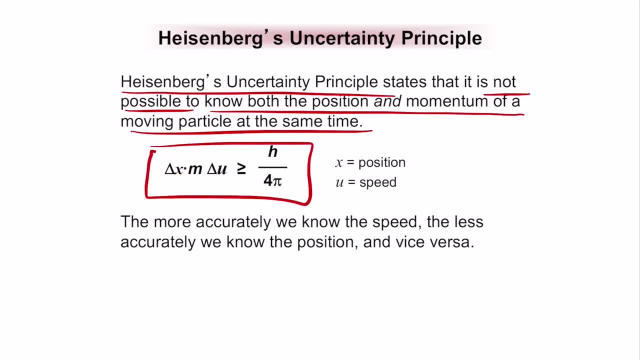 Heisenberg uncertainty equation, which is delta X times m times delta u, is greater than or equal to h by 4 pi, where h is the Planck's constant and m is the mass of the particle. So the more accurately we know the speed, the less 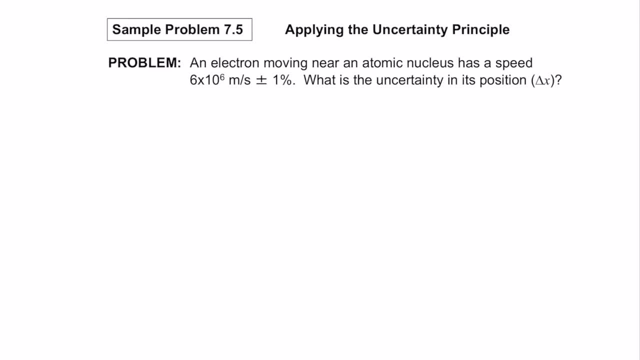 accurately. we know the position and opposite times, y squared. So what is given here? an electron is moving at the same time. at the same time, then it's near an atomic nucleus that has a speed of 6 times 10 to the power, 8 meter per second. 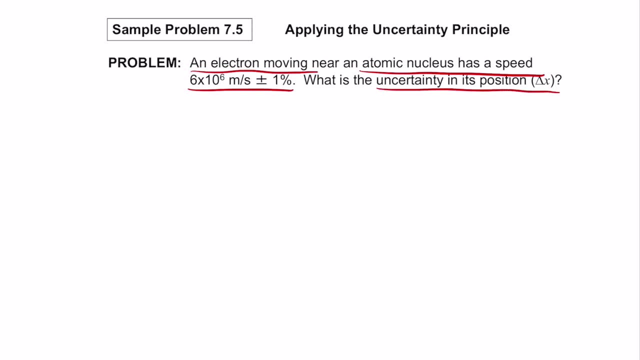 plus or minus 1 percent. what is the uncertainty in its position? so how do you find the value here? so they have given you delta u, which is 1 percent of 6 times 10 to the power 6. so calculate 1 percent, which is 0.01 times 6 times 10 to the. 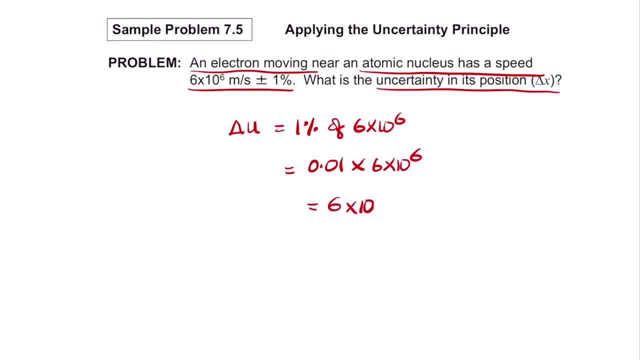 power 6, so which becomes 6 times 10, to the power of 4. so they have given you delta u and they are asking you to find the uncertainty in the position. so we know the formula is: delta x times delta u times m is greater than or equal to h by 4 pi. so delta x is the value that we want, so h greater. 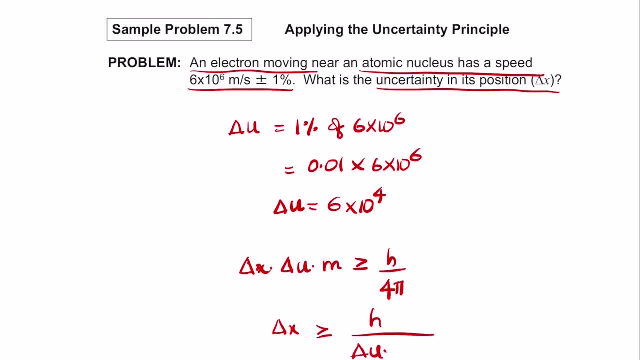 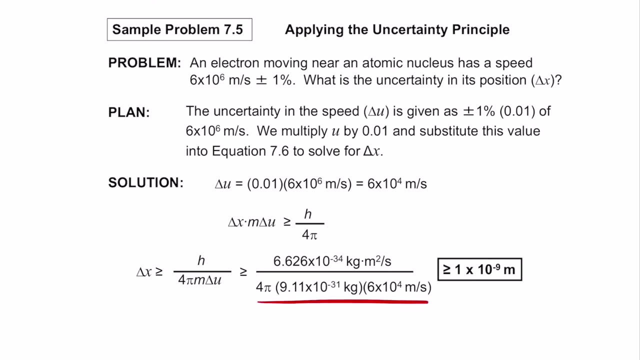 than or equal to h by delta u times m times 4 pi. so substitute all the values and you end up getting you the answer, so that value becomes. so when you substitute everything into the formula, you end up getting an uncertainty of 1 times 10 to the power negative 9 meter. 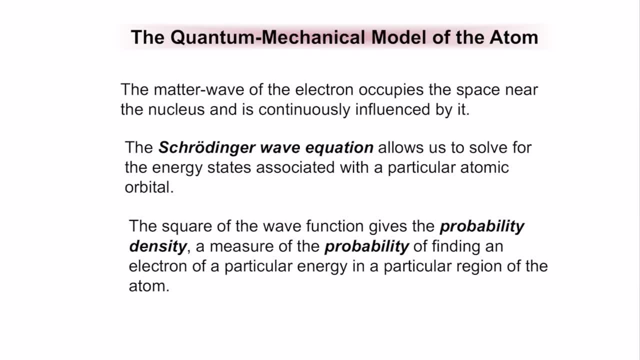 so next let's talk about the quantum mechanical model of the atom, so which was first proposed by schrodinger. so schrodinger basically stated that, rather than a particle being, rather than the electron being at one single place, he said that electron, rather than being at a single place, is generally found in a given region. 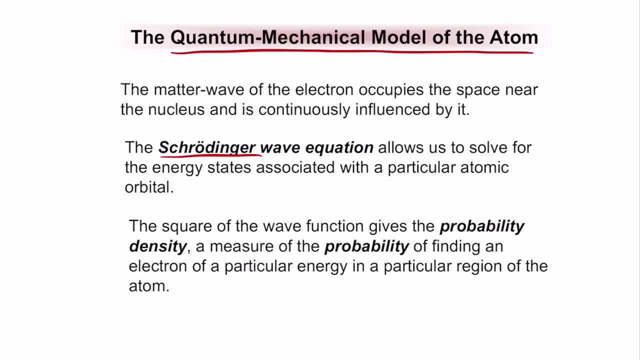 and he said that it's not a deterministic value but a probabilistic value, which basically says that what is the probability or the chance of finding the electron at a particular position? he explained that by using a schrodinger's wave equation which allows us to solve the energy. 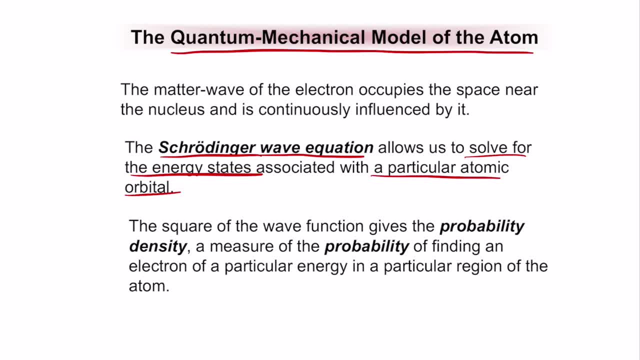 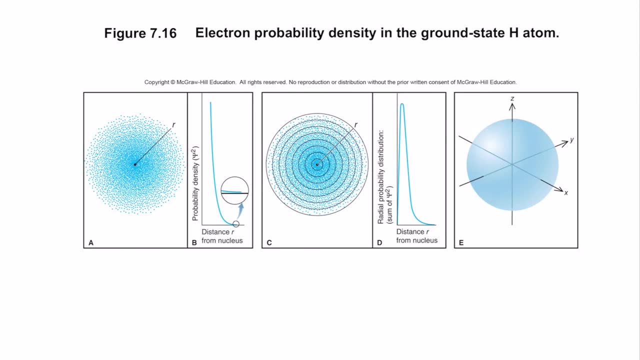 states associated with a particular atomic orbital. so he basically stated that the square of the wave function gives the probability density of the atom and the probability density of the atom and which is the measure of the probability of finding an electron of a particular energy in the particular region of the atom. so for an s orbital, this probability, electron probability. 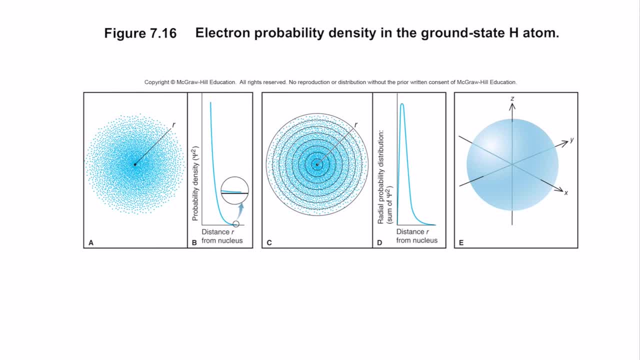 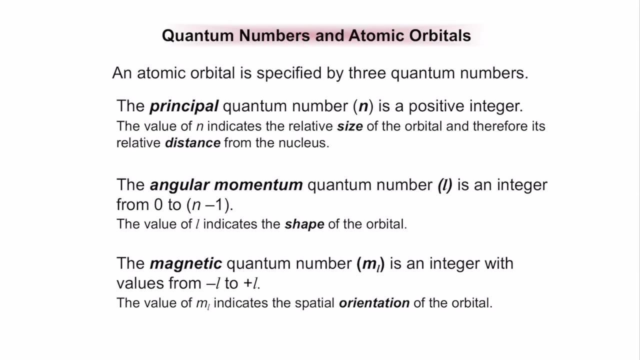 is very high at a single region. so the as you go farther and farther away, the chance of finding the electron becomes lesser and lesser. so this is the s orbitals shape. so this is how we propose the s orbital shape. so the easier way to explain this is by using the quantum numbers and orbitals, atomic orbitals. so 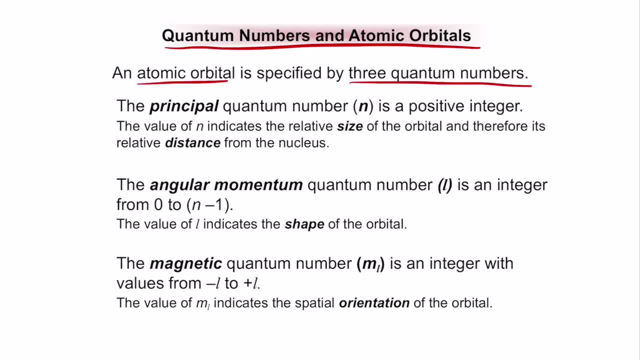 a simple atomic orbital is generally specified by three quantum numbers. the first one is the principal quantum number, which is a positive integer. so the value of the principal quantum number indicates the relative size of the orbital and therefore its distance from the nucleus. second is the angular momentum quantum number given by l, which is an integer from 0 to n minus. 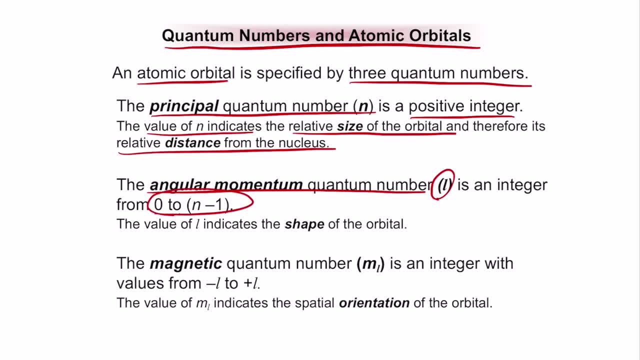 1, so, which is the angular momentum quantum number given by l, which is an integer from 0 to n minus 1, is basically dependent on the principal quantum number and the value of l depends on the shape of the orbital. and the third one is the magnetic quantum number, or m. it is an integer from minus. 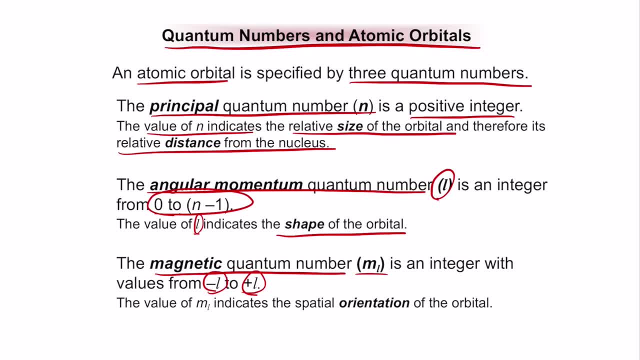 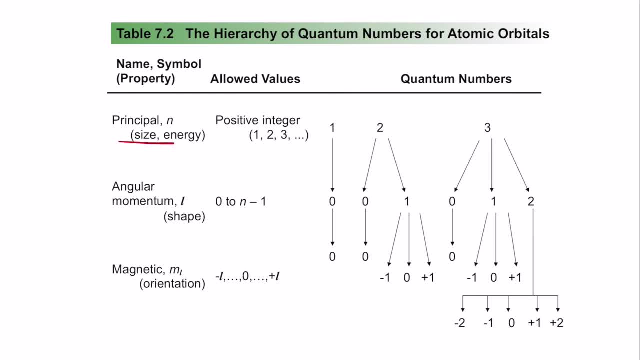 l to plus l, so it depends on the angular momentum quantum number, and the value of ml basically indicates the orientation of the orbital. so for a principle's quantum number of 1, the angular momentum is 0 to n minus 1 so 0, and magnetic momentum is 0 to n minus 1 so 0, and the 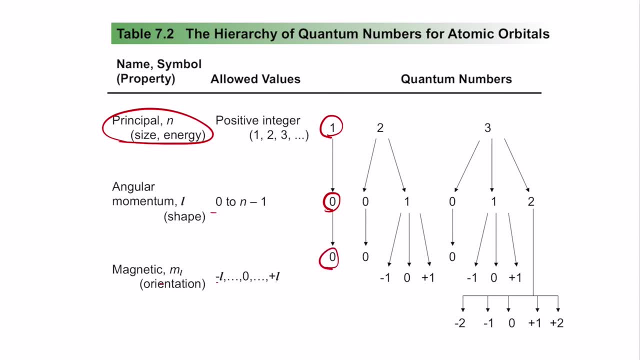 magnetic momentum quantum number is negative L to plus L, so it becomes 0. now for the second principal quantum number. you end up getting two different angular momentum quantum numbers, and for each angular momentum quantum number you get a moment of magnetic quantum number, so which is 0 here. and for 1 you get negative L to L, so minus 1, 0 and 1. in the same way, when you 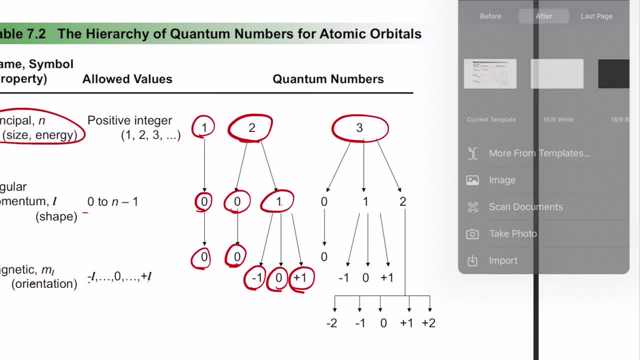 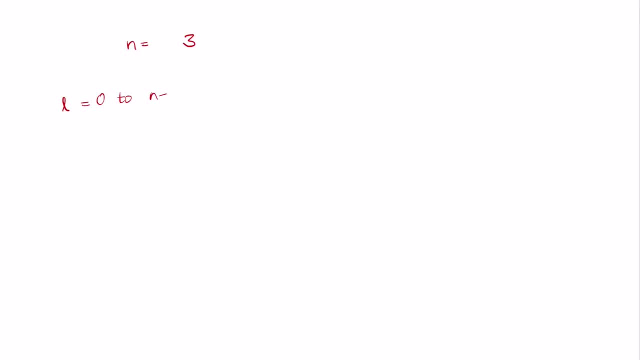 have 3 here, so let me write it down in a separate part. so let's say: if you have 3 here, is n equal to 3, then L becomes 0 to n minus 1, so it can have 0 comma 1 comma 2, so n minus 1 is 2, so it can be. 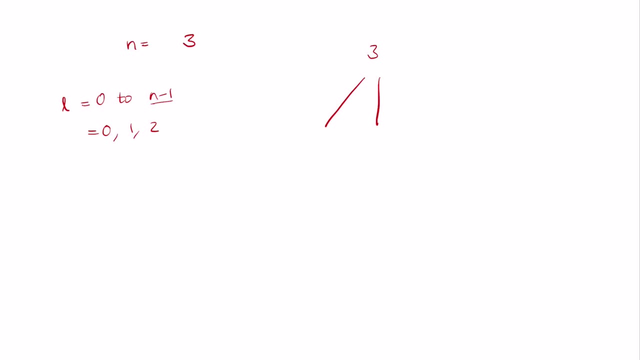 three different values. so from 3 we get three different angular momentum quantum numbers, 0, 1 and 2, and m value stays from negative L to L. so 0 is negative, 0 to 0 is 0 and for 1 you get three. 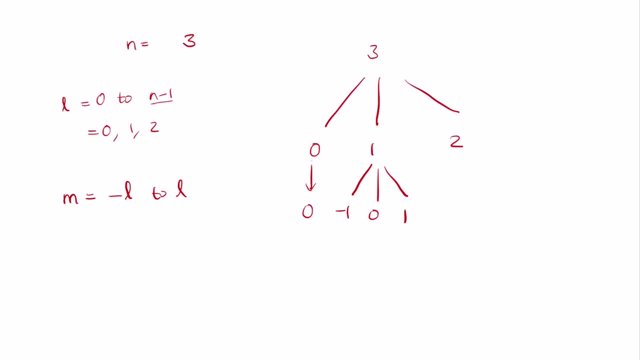 different values, so negative, 1, 0 and 1.. For 2 you get five different values: negative, 2, negative, 1, 0, 1 and 2. so this here represents the n value. this 3 represent the L value and these values represent the m values, ml values. so this: 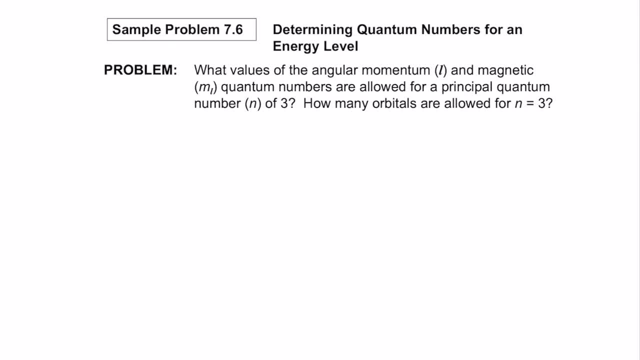 is how you can find the magnetic momentum quantum numbers. so let's say we have what values of angular momentum and magnetic quantum numbers Are allowed for a principal quantum number of n equal to 3 and how many orbits are allowed for n equal to three orbitals are allowed for an equal to three. 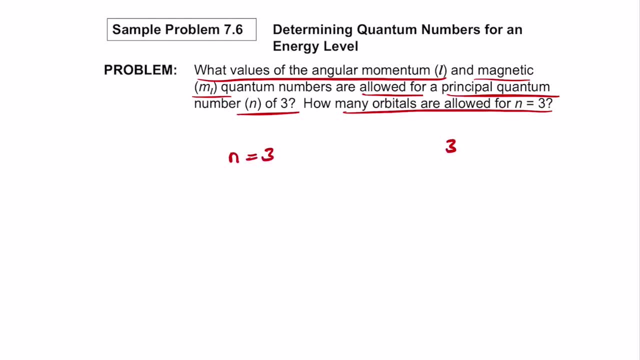 So let's start with n equal to three, so 3. so L is 0 to n minus 1, so 0 to 3 minus one, which becomes zero to 3, 2. Which is basically 0, 1 and 2. so for a principal quantum number of 3, you can have three different. orbitals. So L here represents a random number of 3.. Take one of the three numbers. Remember, before we came to n is m minus m. you can't just write them in one second, so you can write it up and then you can write it down, and then you can also write them in multiple numbers. 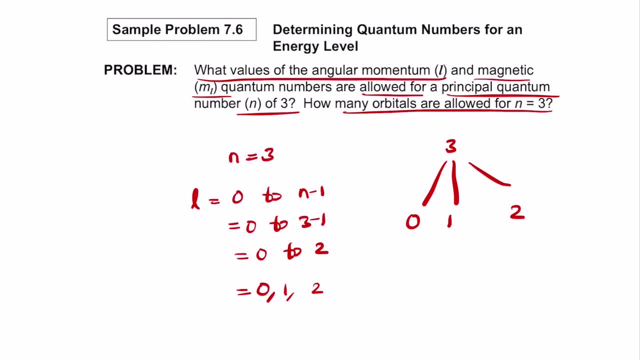 represents the number of orbitals and next for in the magnetic momentum. so each m here is from negative l to l. so notice that there are three different ones. so which means that you start from zero for one, you get negative one to one. so which is negative one, zero one. 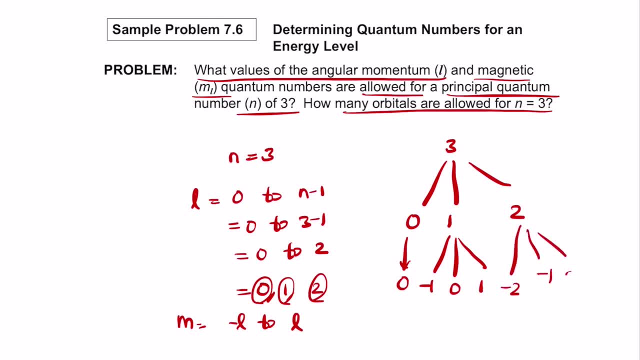 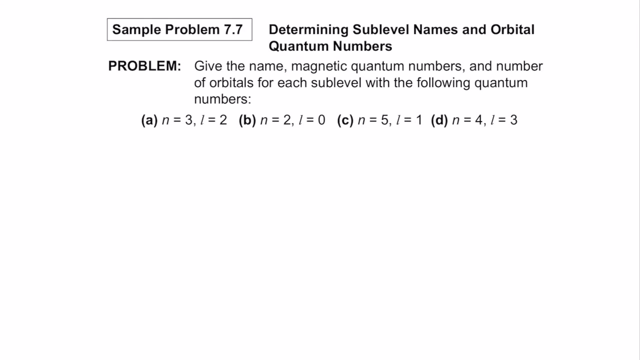 and for two you get negative, two, negative one, zero one, and so this is how we can find the numbers. so use the same principle now. so remember this part. when the depending on the l value, we can also say the orbital. if l value is zero, then the orbital is the s orbital. 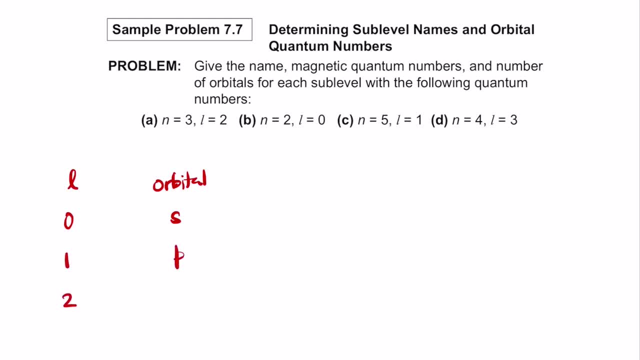 if l value is one, it is the p orbital, if l is two, it is the d orbital, and if l is three, it's the f orbital. so l here represents the orbital. so simply, whenever we want to write the particular position, we can write it there. so n here represents the stock, n here represents the orbit, and l 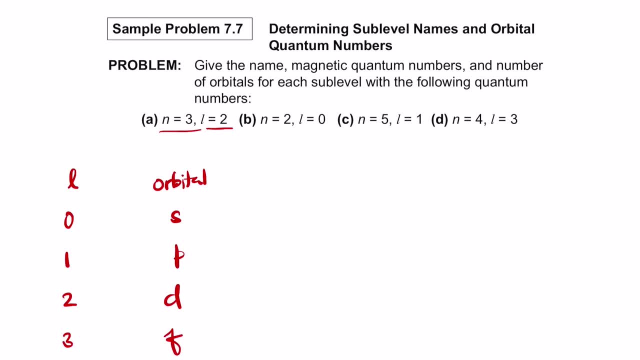 here represents the orbital. so when you want to write the position exactly, so it basically represents that n, l ash, so n and l, we can write it directly. so for example, for the first one, n is three, l is, so for l2, then the orbital is d, so we can write 3d. so because it's 3d, so that we can say that the 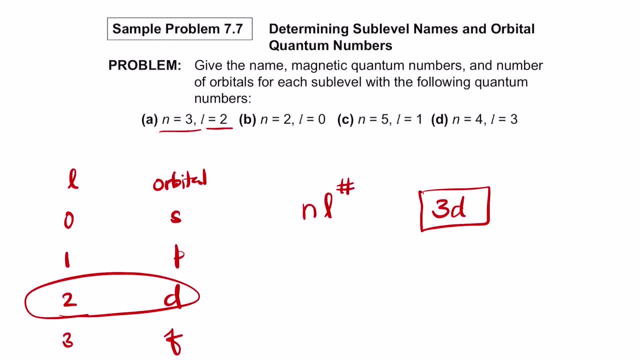 orbital is in 3d and because they are asking us to give the name and magnetic quantum numbers and the number of orbitals for each sub level. now let's try and find for 3d here, when l equal to 2, we know that m is from minus l to l, so which is from minus 2 to 2, so which becomes minus 2 comma. 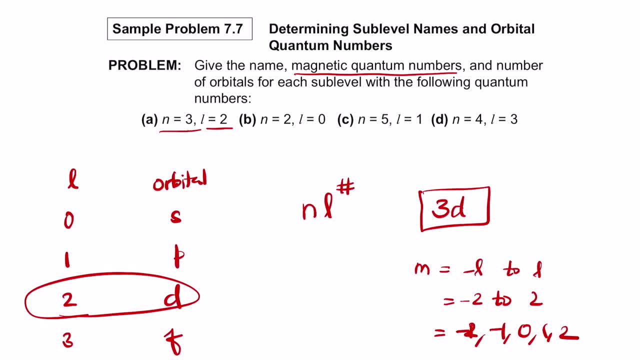 minus 1 comma 0 comma 1 comma 2. so this is the value for m. so this is how we can write. so use the same principle now and write down the rest of the values. so pause the video right here and try to solve the rest of the problems. 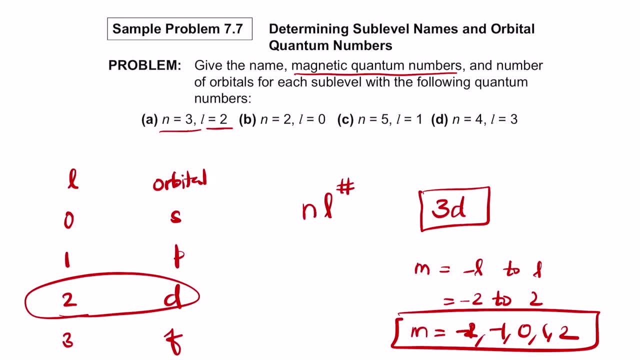 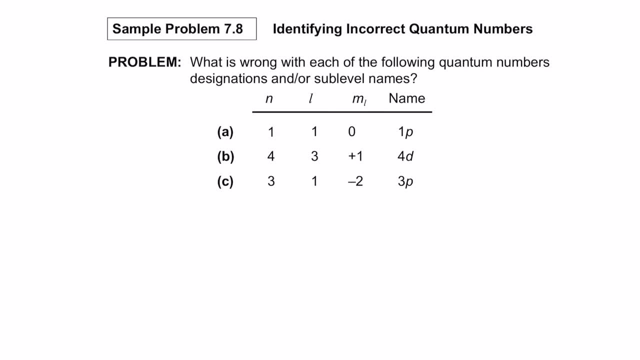 next let's talk about identifying incorrect quantum numbers. so here they have given us n and l and m values. they are asking us to find whether there is a possibility of. if there is anything wrong here, let's take the first one. so when n is 1, so the name is 1. 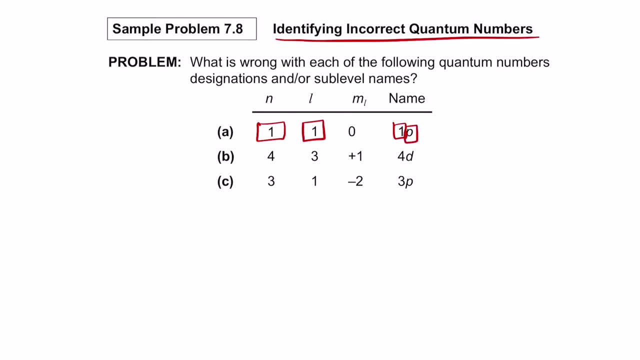 l is 1, so which is p orbital, so 1p. fine, now we know that m here, so notice. the problem here is that when n is 1, l is 0 to n minus 1, so which means 0 to 1 minus 1, so it should be 0. 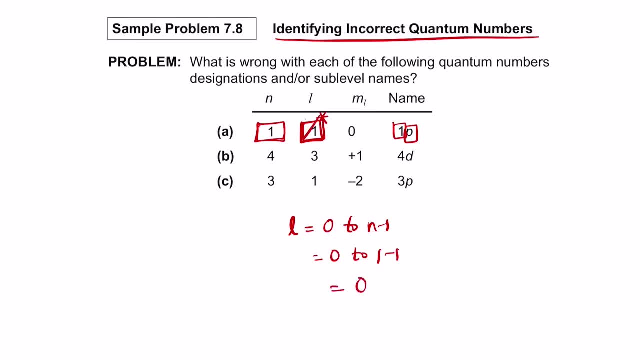 so, which means this is the part that is wrong. so it should not be 1, it should be 0. so, like this, try to find whether the values are correct or not. so try to predict which one of the values that has given here is wrong. pause the video right here and try to solve this problem.